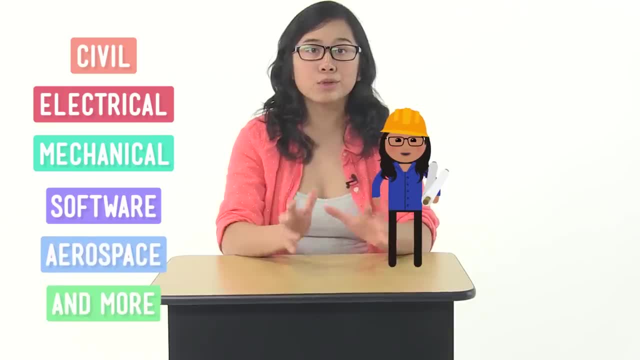 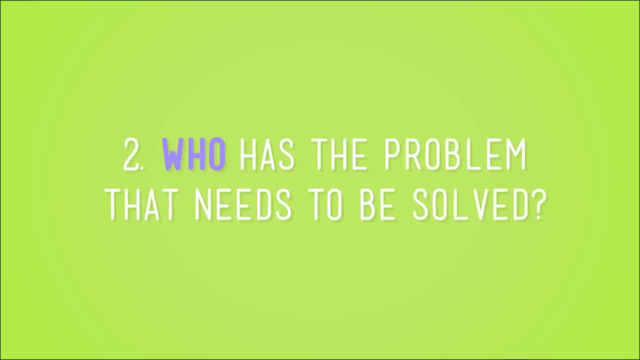 But no matter what type of engineer someone is, they have to ask themselves three very important questions when they're working. Number one: what is the problem that needs to be solved? And number two: who has the problem that needs to be solved? 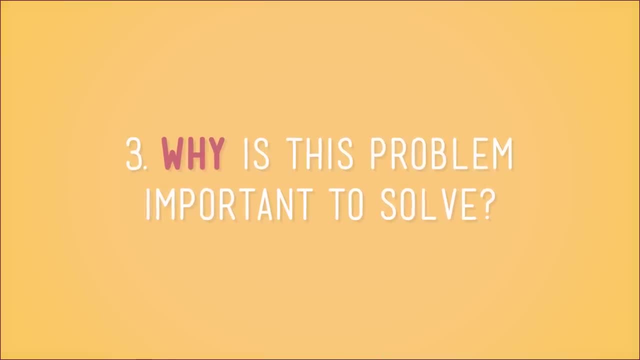 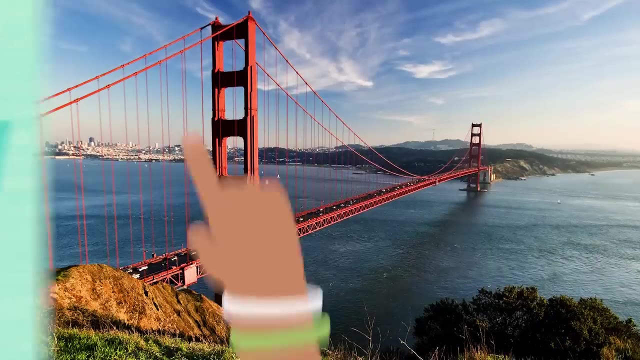 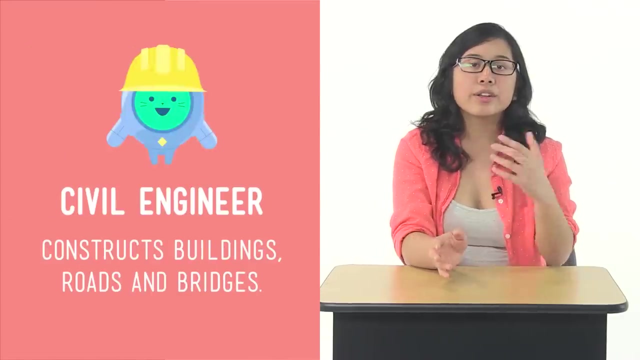 And, most importantly, number three: why is this problem important to solve? Let's take a look at some examples. A really famous example of engineering is the Golden Gate Bridge in San Francisco, California. I mentioned that there are different kinds of engineers, and a civil engineer is someone. 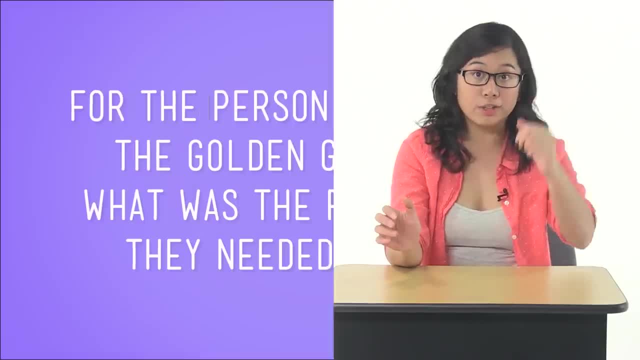 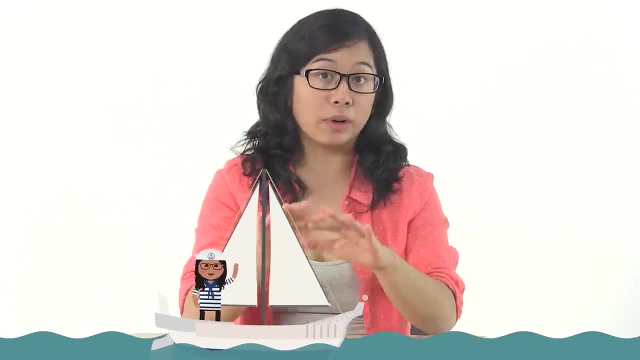 who designs and constructs buildings, roads and yup bridges. For the person who designed the Golden Gate Bridge, what was the problem that they needed to solve? People couldn't travel in or out of San Francisco, which is surrounded on most sides. 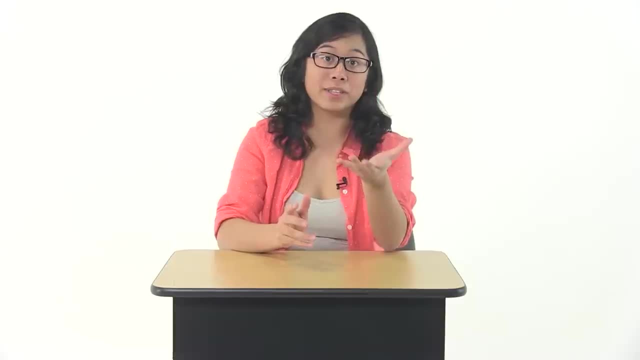 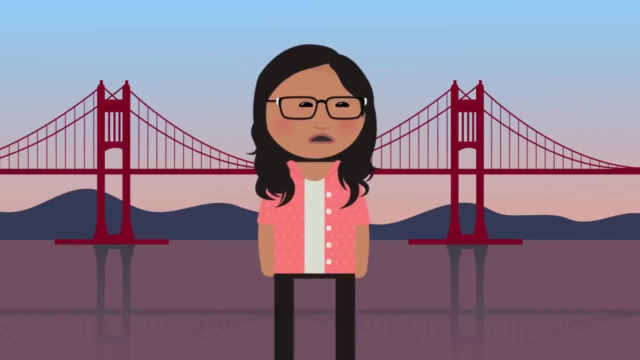 by water without a boat. Who had the problem? Residents of San Francisco, San Francisco mostly, but really anybody traveling in the area. And why was the problem important to solve? Well, you didn't want a whole bunch of San Francisco residents trapped in San Francisco. 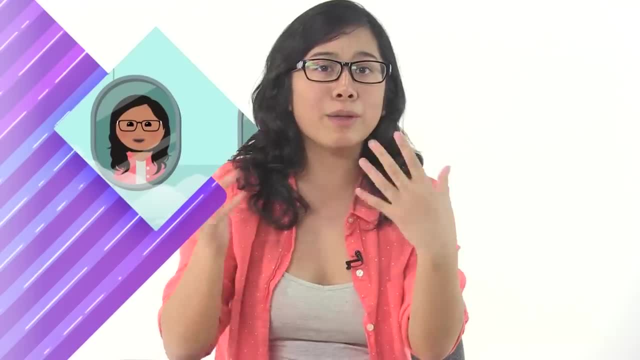 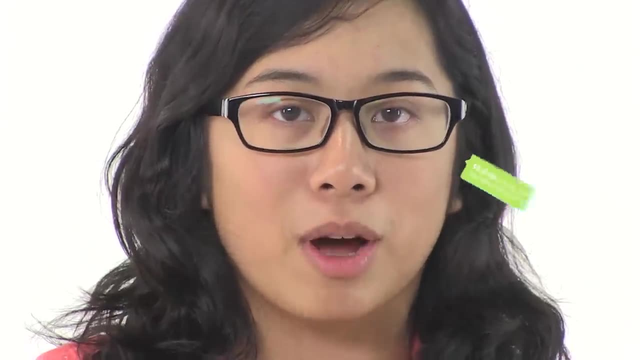 forever, even if it is a super cool city. Plus, you wanted people outside of San Francisco to be able to travel to the city easily if they needed to, So the Golden Gate Bridge was engineered as a solution to this problem. In addition to civil engineers, there are also mechanical, electrical, chemical, computer. 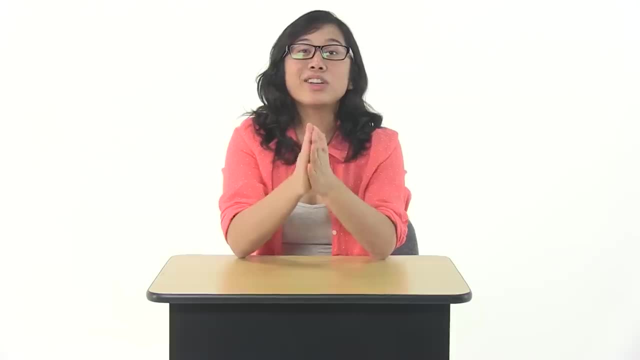 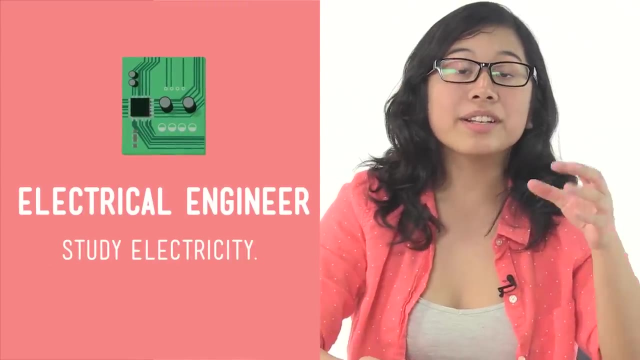 nuclear and software engineers, and the list goes on. Let's talk about what some of the other types of engineers did. First up, electrical engineers. Electrical engineers study electricity. they design electrical systems like circuits and computer chips. Think of an electrical object that you use pretty regularly. 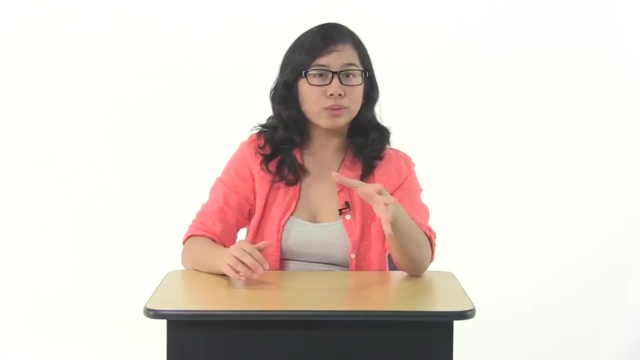 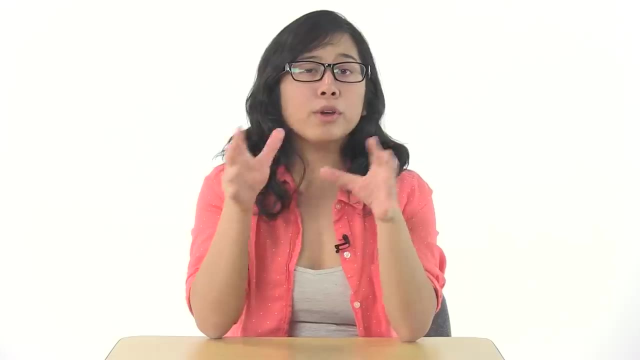 How about your microwave? What problem was the microwave? a solution to Cold food, right? You have an electrical engineer to thank for the ability to reheat that leftover pizza you just had for lunch. But while you might not have heard of Joseph Strauss or Percy Spencer, the engineers responsible, 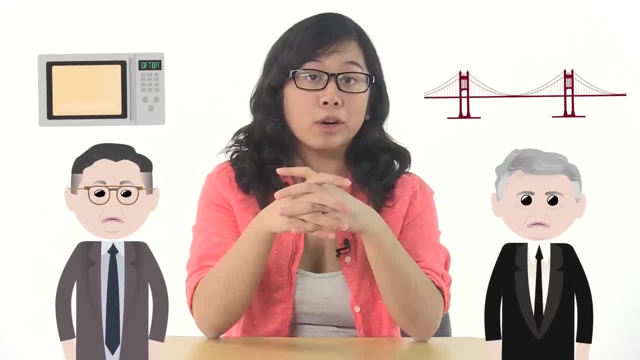 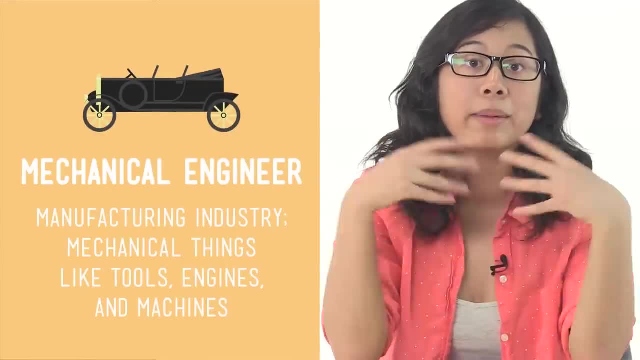 for the Golden Gate Bridge and the microwave respectively. you've probably heard of Henry Ford. Do you know any Ford cars? Henry Ford was a mechanical engineer or someone working in the manufacturing industry making mechanical things like tools, engines and machines. 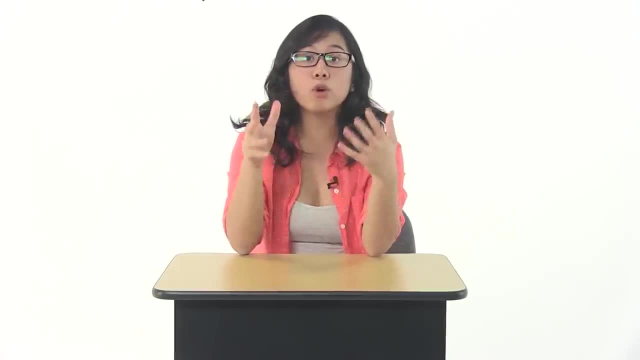 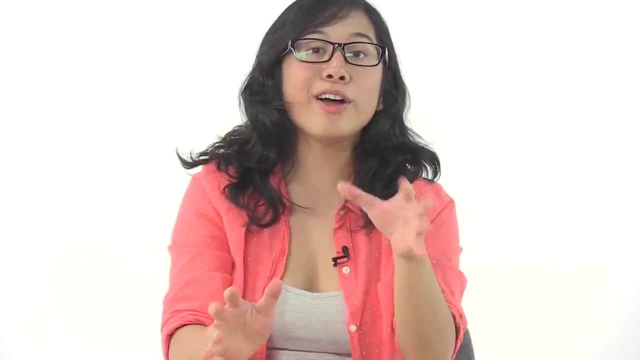 Machines like cars. Ford didn't invent the automobile, but his Ford Motor Company made a lot of them. His Model T car was famous for being affordable for plenty of Americans. Ford saw that lots of people who wanted to drive cars just couldn't. because they couldn't. 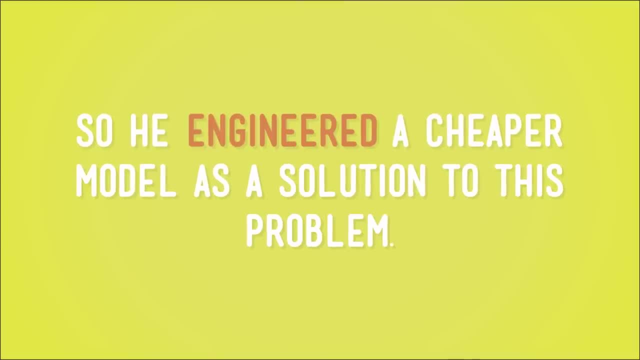 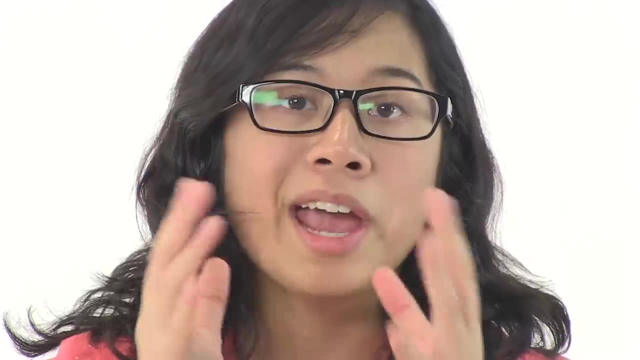 afford the pricey vehicles that were for sale. So he engineered a cheaper model as a solution to this problem. His fellow engineers started to build cars, They started to do the same and now, well, cars are everywhere. Henry Ford's not the only big-name engineer. 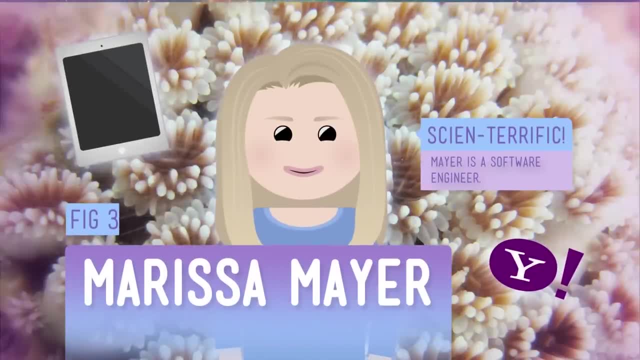 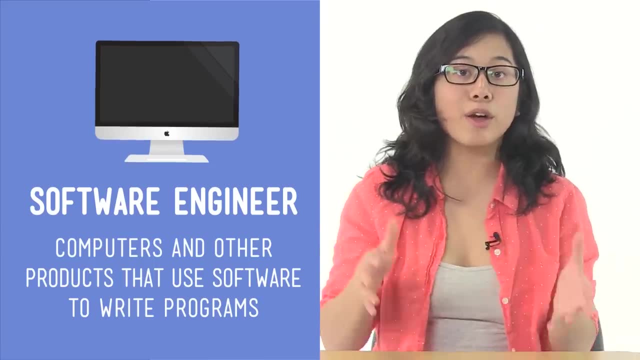 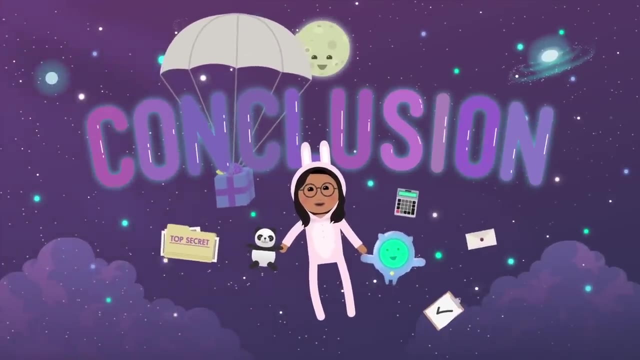 A famous engineer around today is Marissa Mayer. Mayer is the president of the internet company Yahoo and is also a software engineer. Software engineers work on computers and other products that use software to write programs to make them faster and able to do more things. 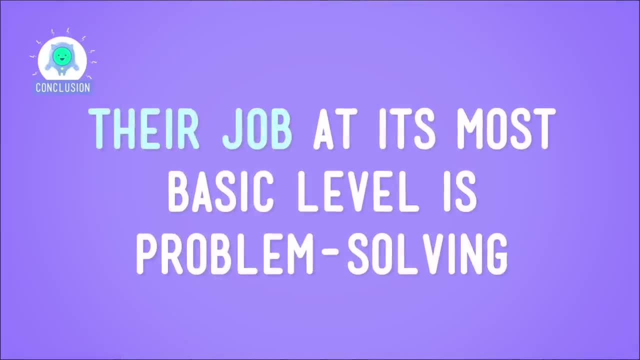 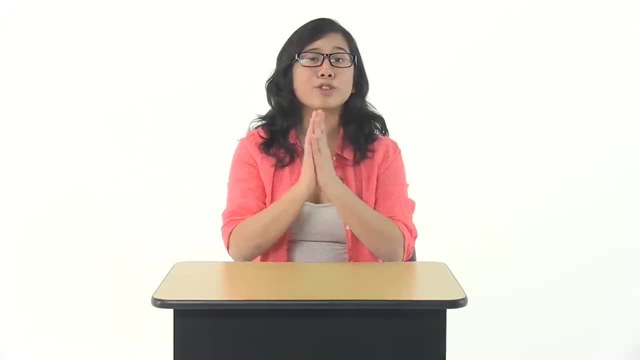 No matter what kind of engineer someone is, their job at its most basic level is problem-solving. Each engineer just specializes in solving certain kinds of problems, While it might seem like there are too many types of engineers to keep track of just wait fifteen years, Or fifty, Or one hundred, Because we'll probably have a ton of different types to add to the list by then. Think about it: Over a hundred years ago, we didn't have jobs in fields like aerospace engineering, where people design and construct planes and spacecraft. 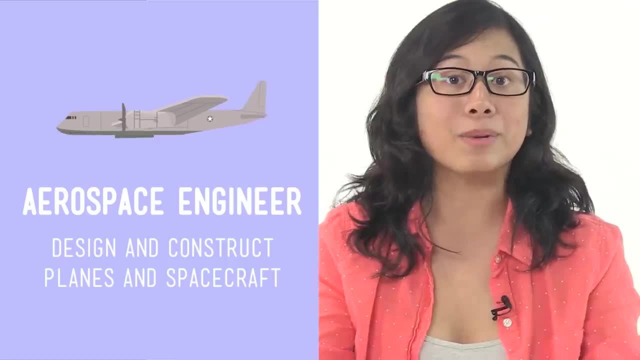 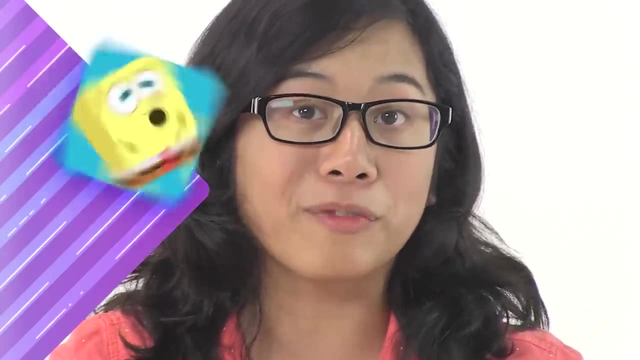 We didn't have planes like we do today or need spaceships, so we didn't need people to engineer them. Who knows what machines or tools or everyday objects or things like that can be used to solve problems? We don't know how many projects we'll have in the year 3015,. personally, I'm hoping. 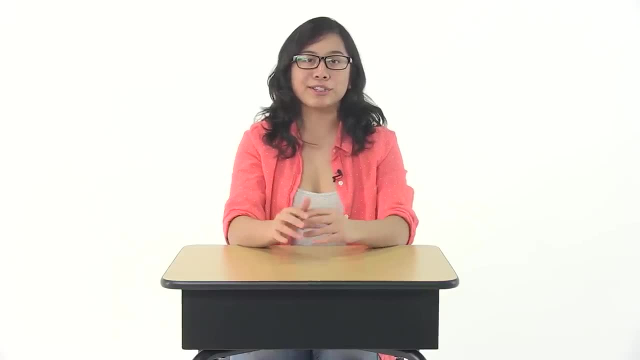 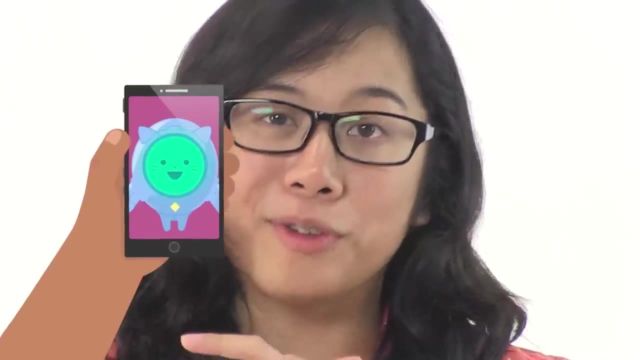 for underwater cities. But whatever these things are, we'll need engineers to make them. So what do you say? Who wants to be an engineer? I'm going to take a wild guess and say you've probably used a phone And I bet you've enjoyed the benefits of a little thing we call air conditioning. 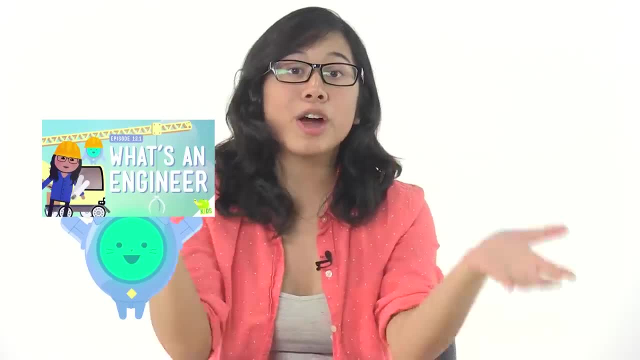 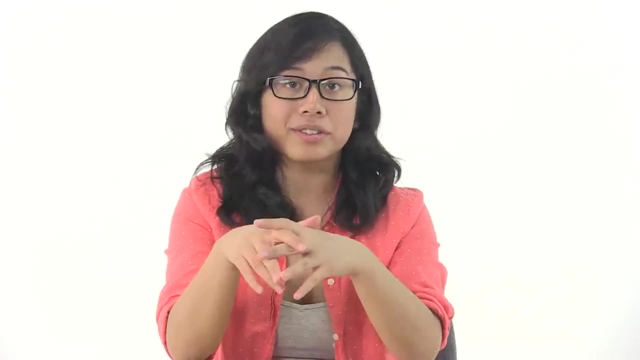 You know who made those things possible? Engineers. We were just talking about engineers in our last video, people who design and build things to solve problems, and there are lots of different kinds of engineers. No matter what type of engineer you want to be, though- civil, mechanical, electrical. 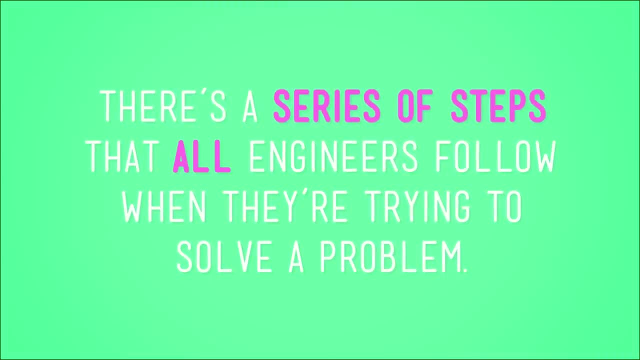 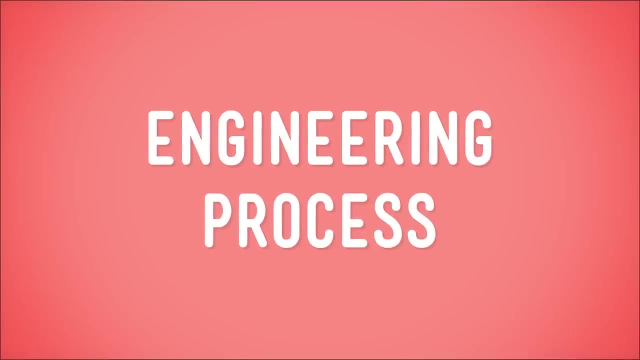 or a kind that doesn't even exist yet. there's a series of steps that all engineers follow when they're trying to solve a problem. This process is called wait for it. the engineering process Makes sense to me. So what sort of steps are included in the engineering process? 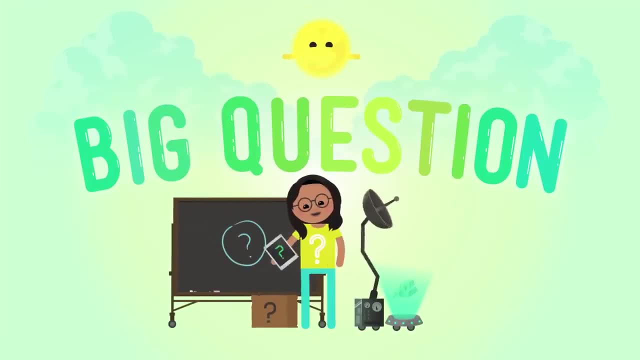 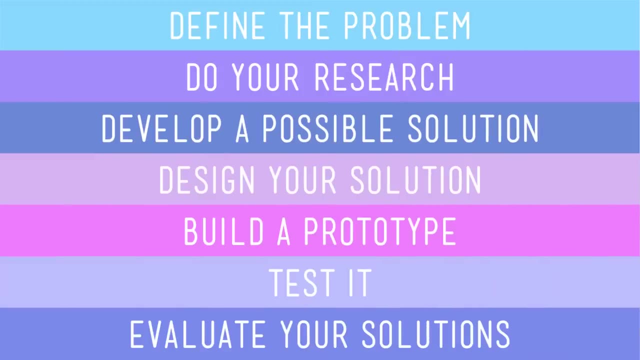 And why do we need it? Let's go through it step by step and discover how awesome things are made. First thing you gotta do is just define the process, And that's what we're going to do. I mean, before you can solve a problem, you have to figure out what it is right. 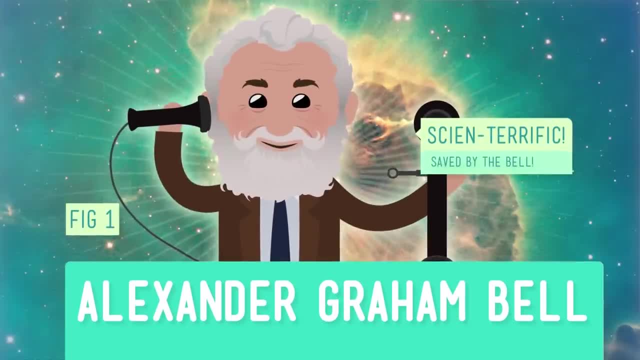 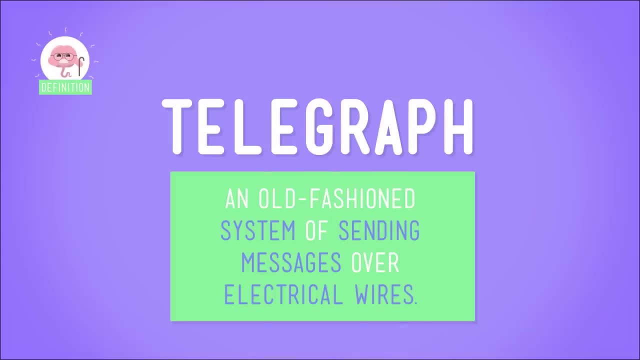 For example, back in the 1800s, an engineer named Alexander Graham Bell was trying to come up with a simpler, cheaper way for people to communicate. Back then, the best you could do was a telegraph, which was an old-fashioned system of sending. 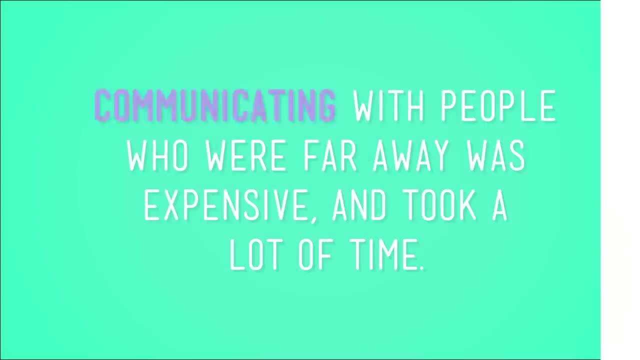 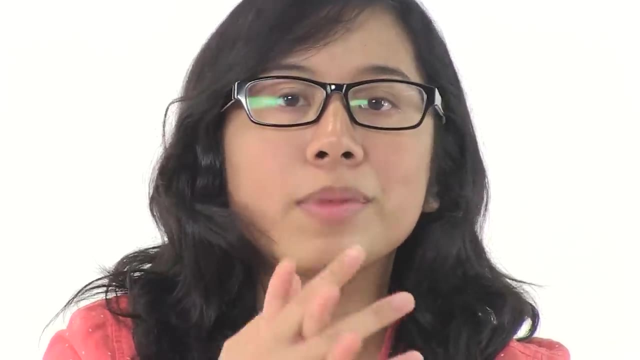 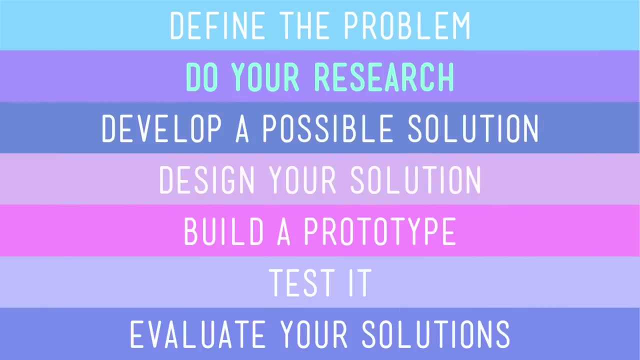 messages over electrical wires. Bell identified his problem: Communicating with people who were far away was expensive and took a lot of time. So his invention or solution to this problem was something you may have heard of: The telephone, Nice. But once you've figured out what problem you want to tackle, you need to do your research. 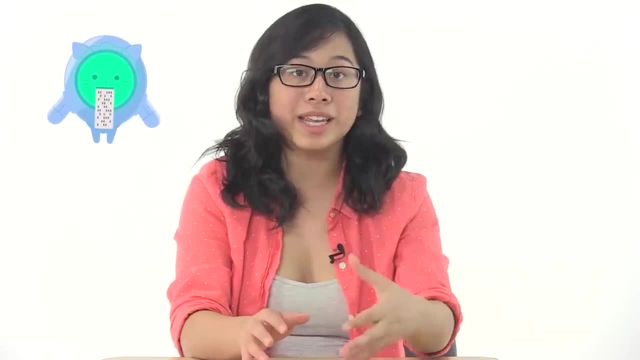 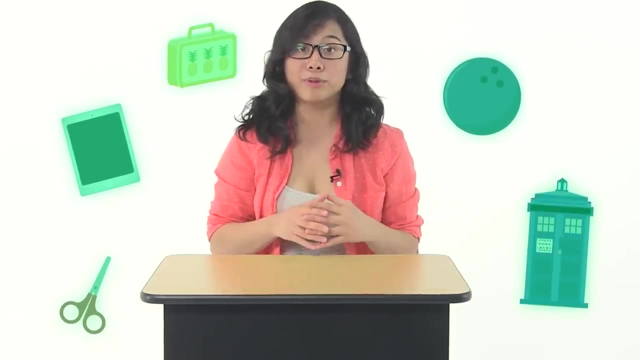 You can start by just making a list of questions you have and what information you need to start answering them. You can also look around and find what other things already exist that have tried to solve this same problem. Maybe they can be improved. A good example here is the man who helped us blow stuff up. The chemist and engineer Alfred Nobel invented the explosive known as dynamite, not because he particularly enjoyed explosions, but because miners and other people who well needed to blow stuff up to do their job, They needed an explosive that was safer to use. 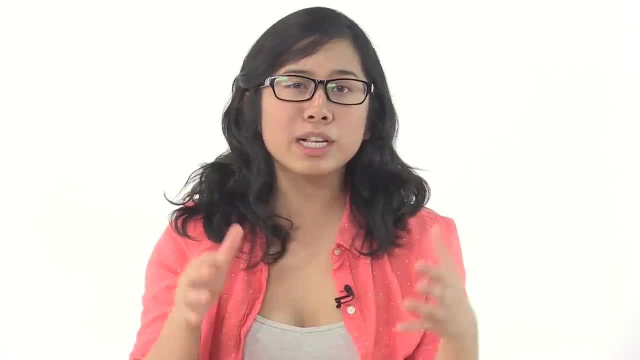 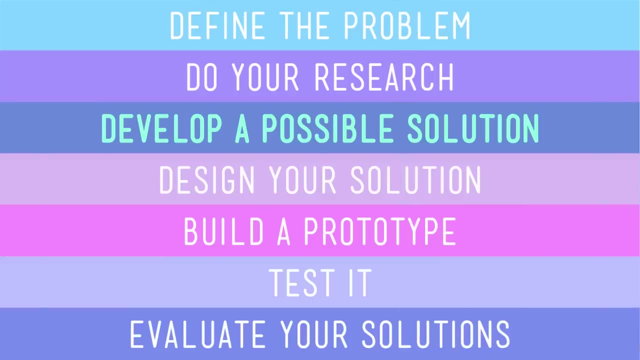 So before he started on that problem, Nobel did research to see what explosives already existed, which ones worked well and which ones didn't. This takes us to step three: develop a solution After your research is done. this is where you say exactly how you think you can solve. 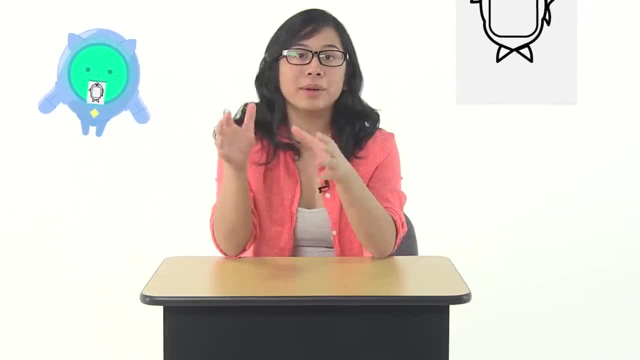 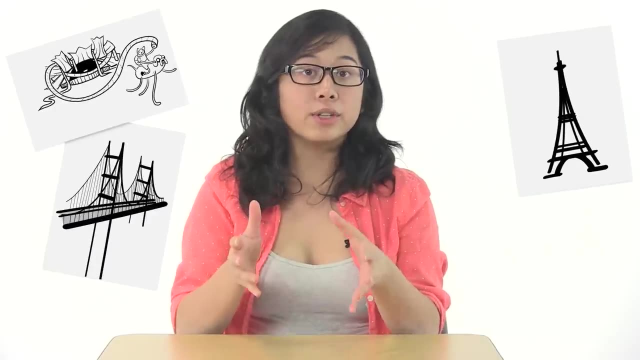 the problem. And once you've thought of a good solution, you have to figure out how it'll actually work and what it will look like. So you have to design your solution. This is where you get to draw. Civil engineers always sketch out their ideas. 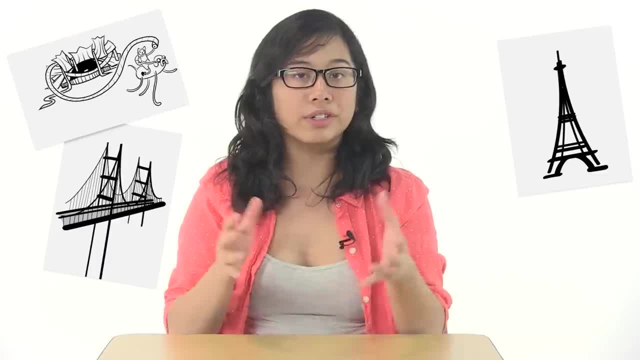 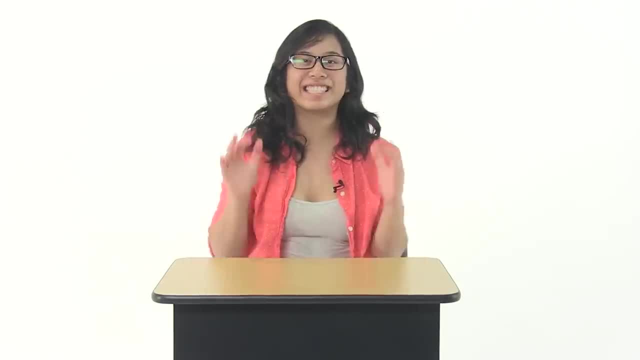 Like buildings and bridges and towers to show what they'll look like when they're done. Gustave Eiffel designed the famous Eiffel Tower in France and he definitely showed up on day one of construction knowing exactly what it was going to look like. 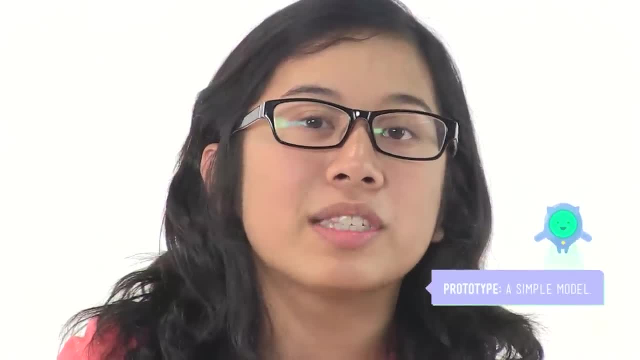 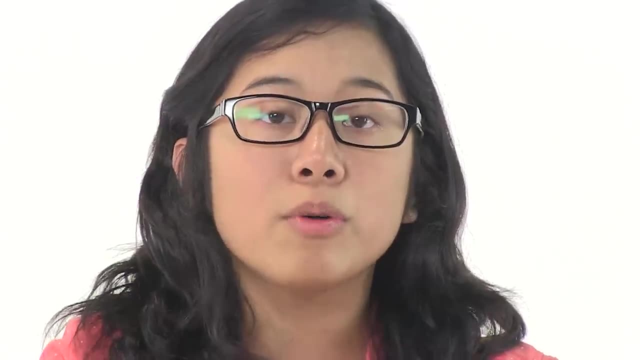 On to step five: build a prototype. A prototype is just a simple model that lets you test out your design. It can be as big as the real thing's going to be, or it can be a smaller version. You just need to have a prototype so you can test it. 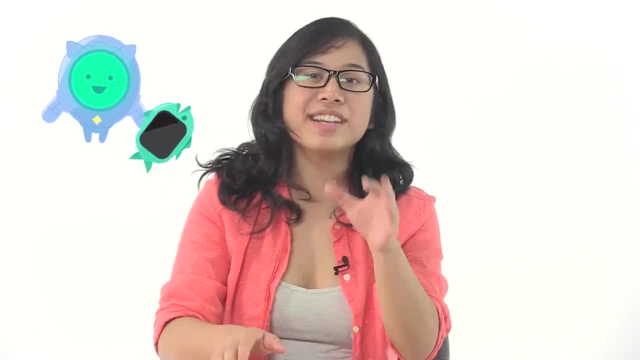 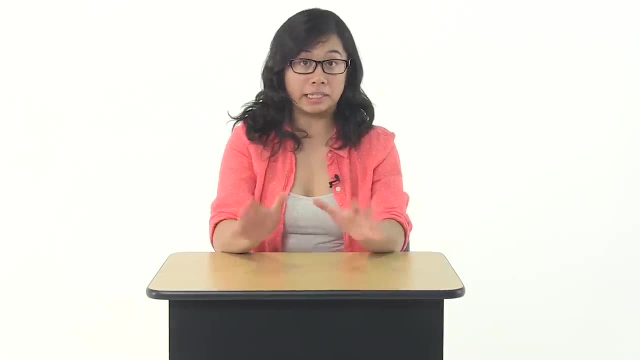 This may be the most important step in the whole process. Engineers need to test their design to see if it works like they want it to. So say, if your building's a big tower, does it stand up? Does it stay standing up? 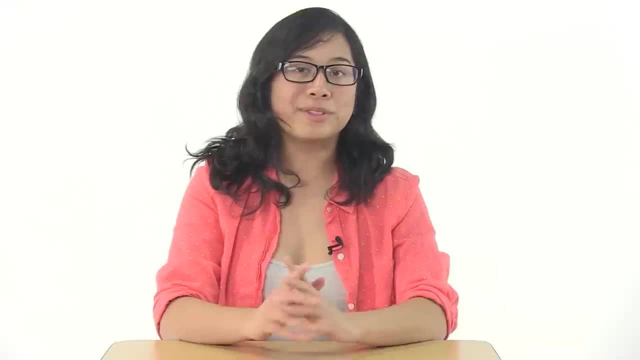 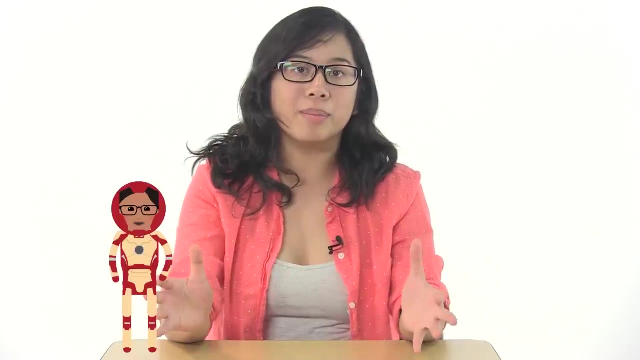 If you're designing something with moving parts, does it work the way you want? Now take it from me, my future engineers. you might have a great idea, a really terrific solution to a really big problem, But when you get to this step, your prototype probably won't work exactly the way you. 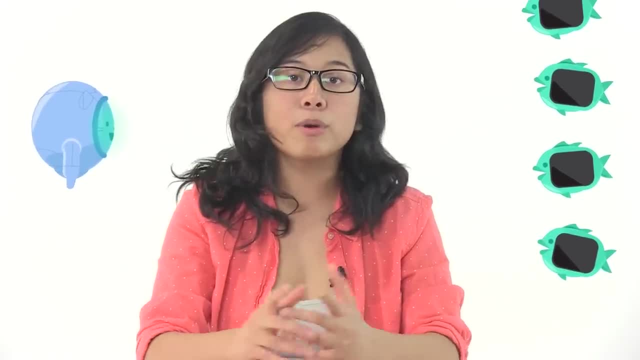 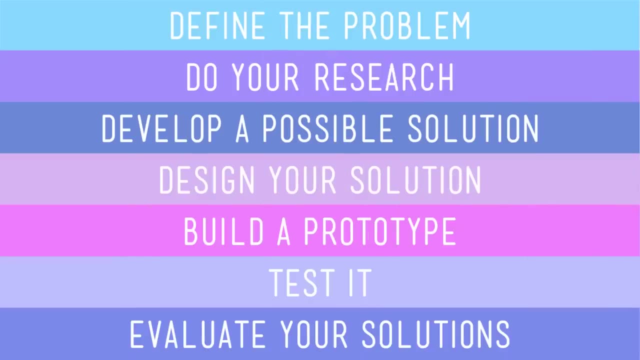 want, At least not on the first try. Most engineers test their prototypes over and over and over again. Most engineers test their prototypes over and over and over again. Most engineers test their prototypes over and over and over again. That's why a lot of time and brainpower goes into the very last step. 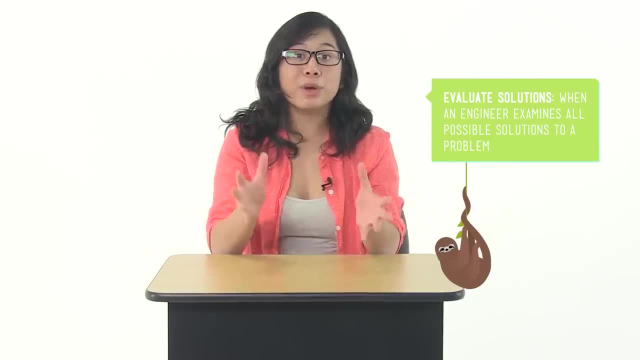 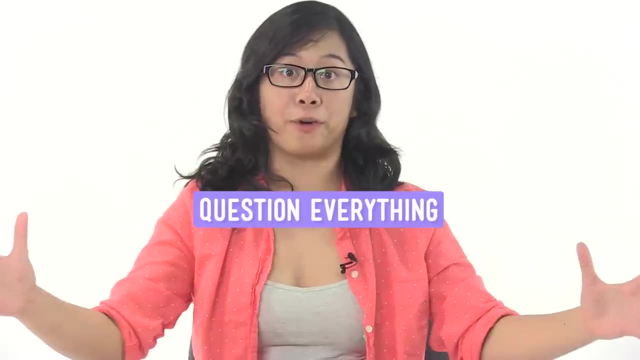 Evaluating your solutions. Evaluating just means asking yourself whether things are working the way you want, or why they are or aren't. I like to think of this step as question everything. This is when engineers review all of the facts and ask themselves questions followed by 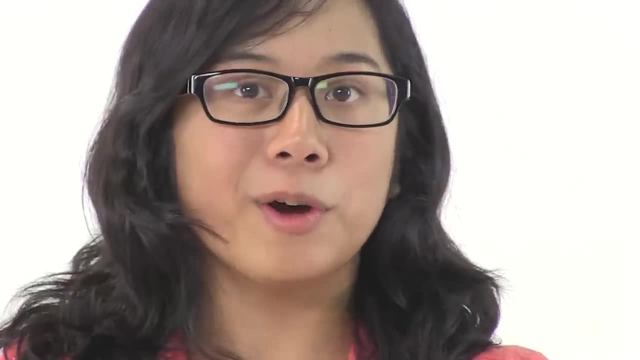 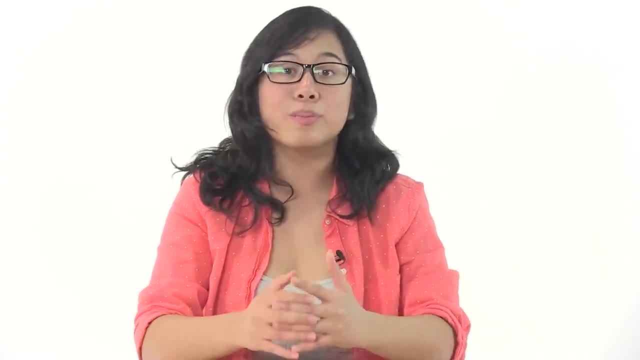 even more questions: What worked well? Why did it work? Why didn't it work? How could it be made better? And most of the time, the answers to these questions are going to send you back several steps, Like. once you figured out why your prototype wasn't working, you'll have to design. 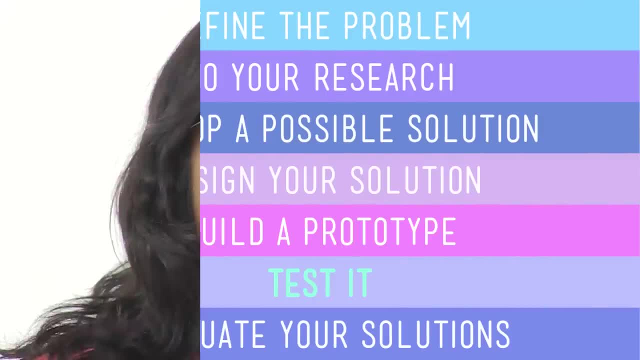 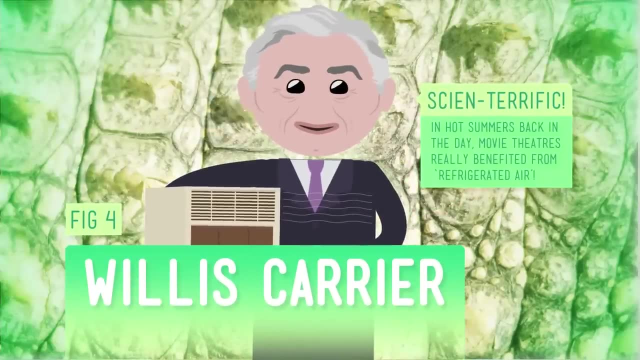 a new solution and then build it and then test it again. Sometimes engineers go through this process four, five, even six times or more. Take Willis Carrier, the inventor of modern air conditioning. He tested his prototypes for years before he figured out the design that worked. the 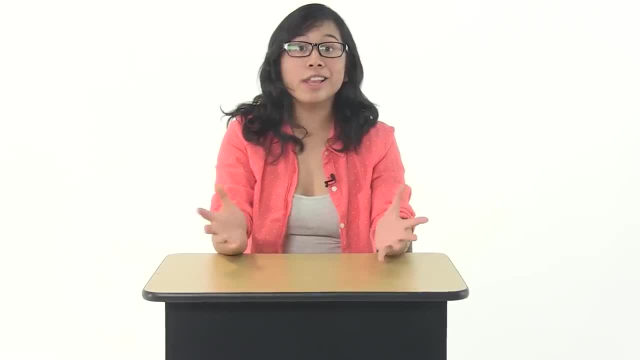 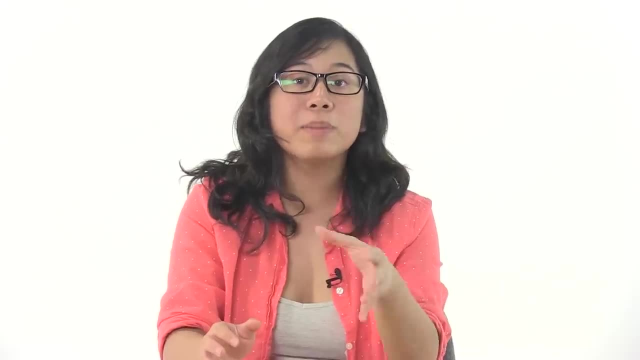 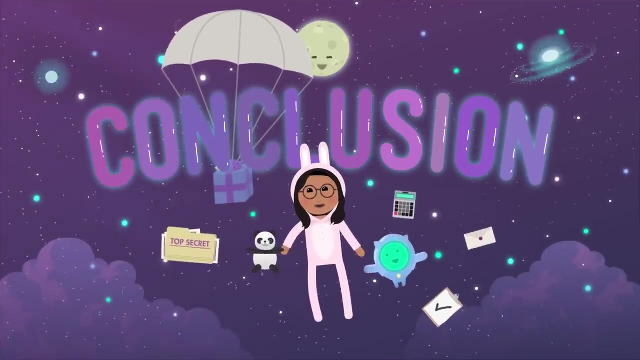 way he wanted and solved the problem he wanted to fix. Like all engineers, he failed. He failed a lot before he succeeded, And that's okay, because he learned something from every failure which made his product even better in the end, And I for one am glad he kept going. 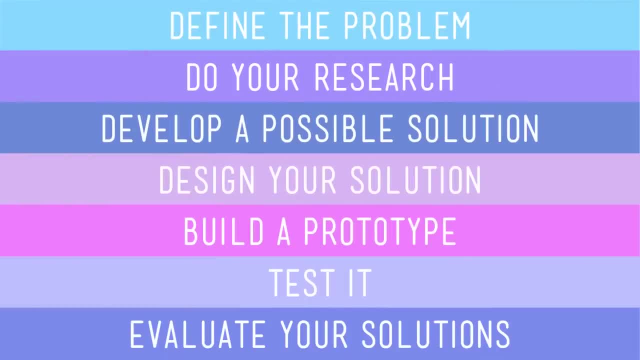 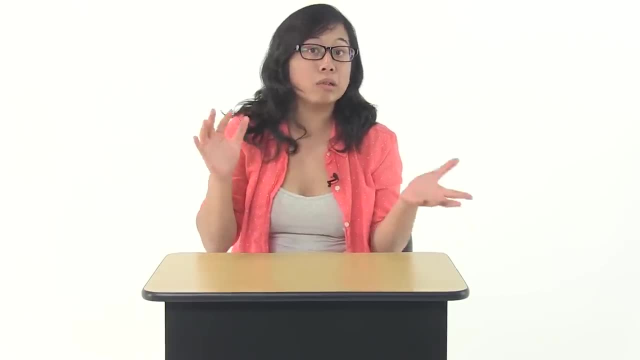 So the engineering process is a series of steps that engineers, or anyone, should use when they're facing a challenge. The process is important because it allows engineers to experiment and also to fail. Both of these things give engineers a chance to go back and improve on their original projects. 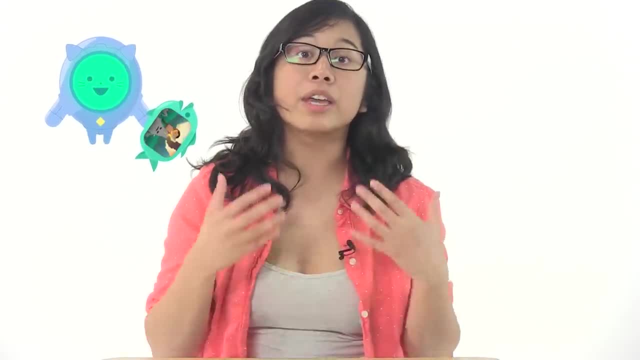 And that's why we're here today. We're here to help you, To give each one of you success, To help you guys out this week. And that's all we have for you today, And we hope you liked those enterprises too. 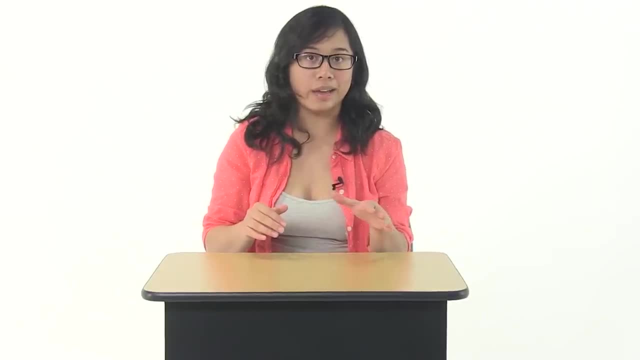 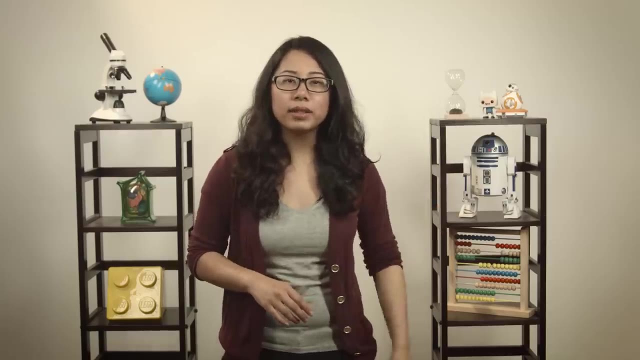 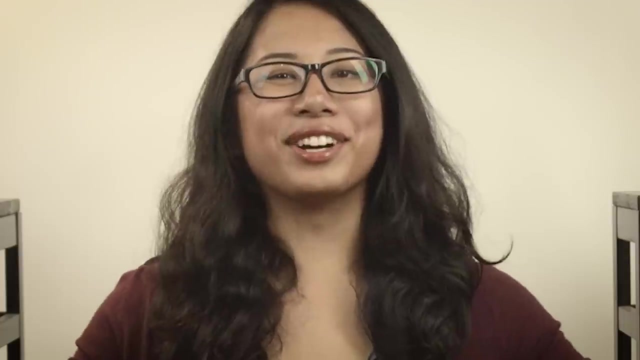 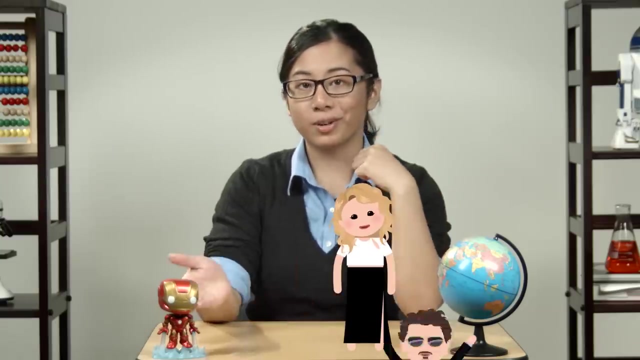 But in the meantime I hope you enjoyed your first of two episodes of The που grid and something wonderful is coming up in the next few weeks. Bye for now, Bye, Bye, Bye might seem like a pretty big deal to you, but when you compare them to other bigger problems, 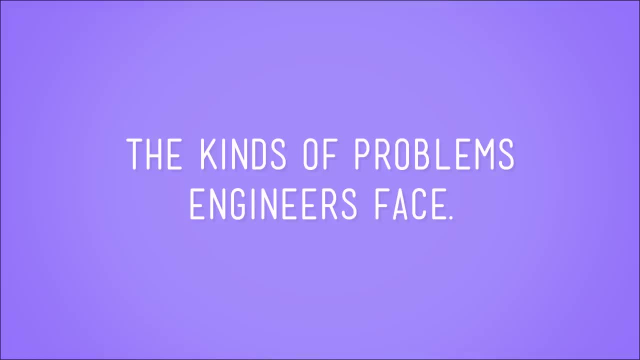 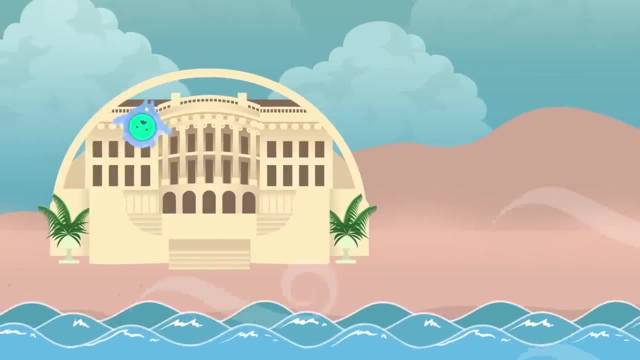 they're really not so bad. Like what kind of bigger problems? Well, the kinds of problems engineers face, like how to safely fly hundreds of people through the air in a small vehicle from one country to another, or how to make an eco-friendly building in a seaside town, that 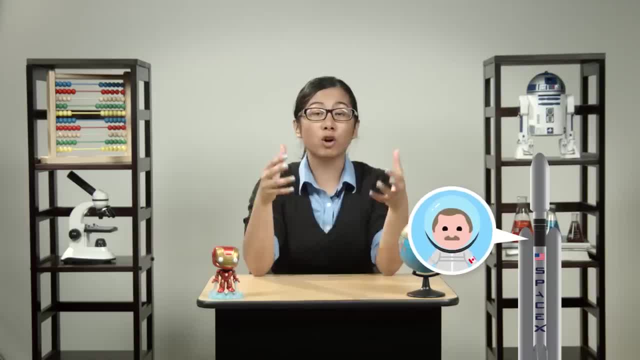 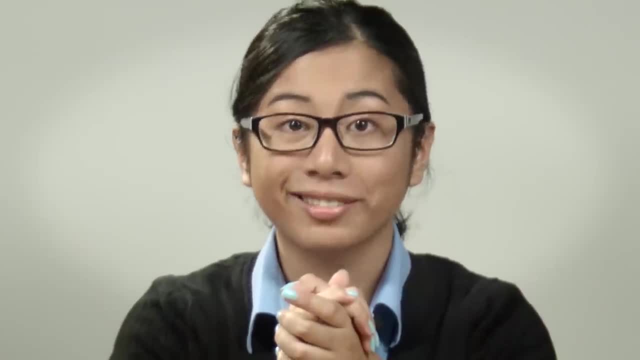 can withstand hurricane, force winds or how to send a bunch of earthbound humans hurtling off into space and, you know, get them back. That homework doesn't seem like such a big problem anymore, does it? Okay, to be clear, I'm not saying that you don't have to do your homework. 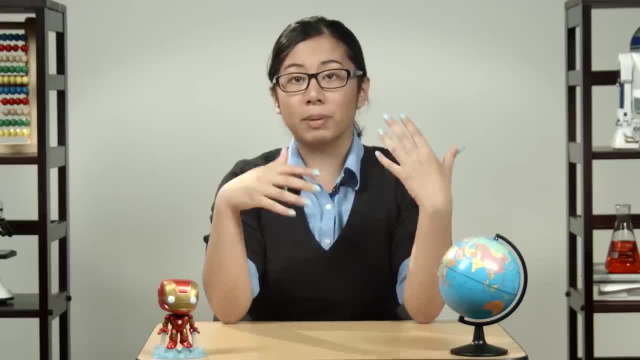 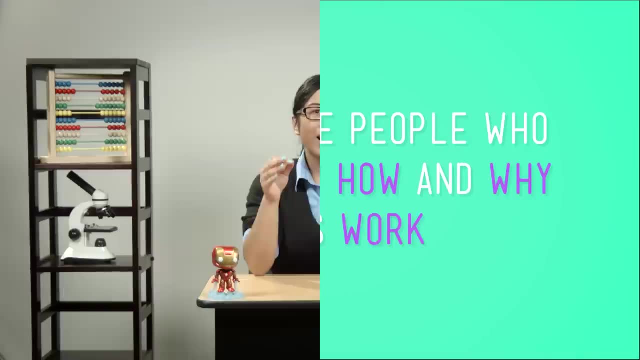 If you didn't, it would definitely be a problem, just not as big as like having to invent a spaceship, And that's the kind of stuff that engineers do. Engineers are people who want to know how and why things work. Not only that, they actually design and build things like machines, systems or 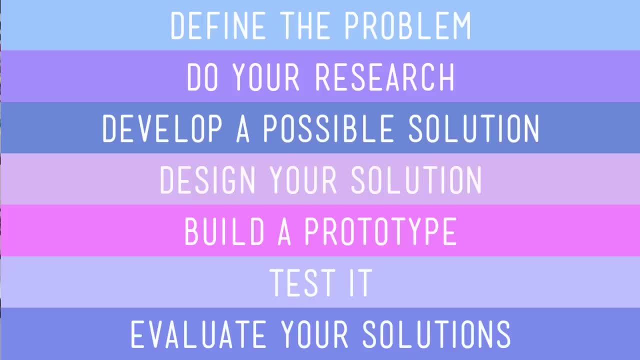 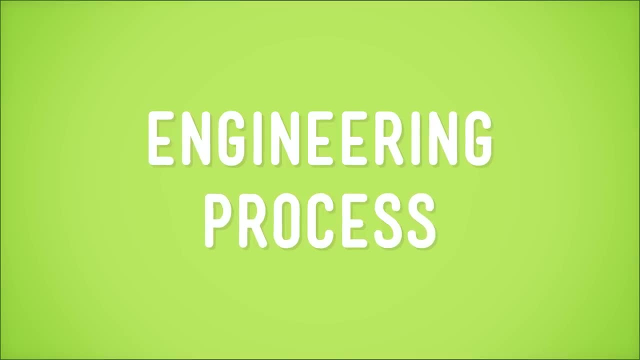 structures to help solve specific problems. All engineers, whatever type they are, follow the same series of steps when trying to solve a problem. You'll remember these steps as the engineering process, and the first step in that process is defining the problem. when an engineer identifies a problem he or she hopes to solve, 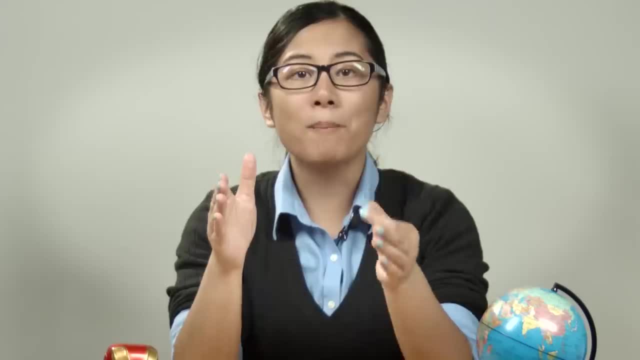 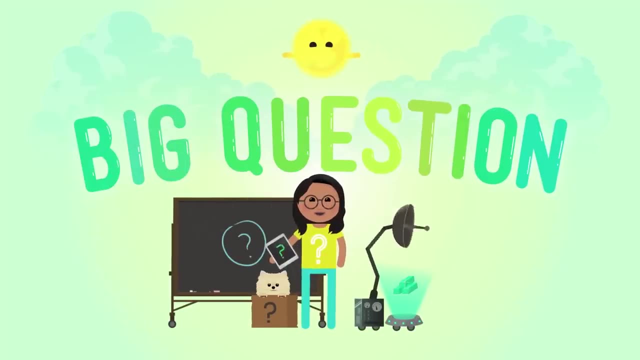 But that first step isn't as simple as you think it is. So it's time for our big question: How does an engineer define a problem? Let's come up with a fake problem to solve, and we'll see what we wind up with. 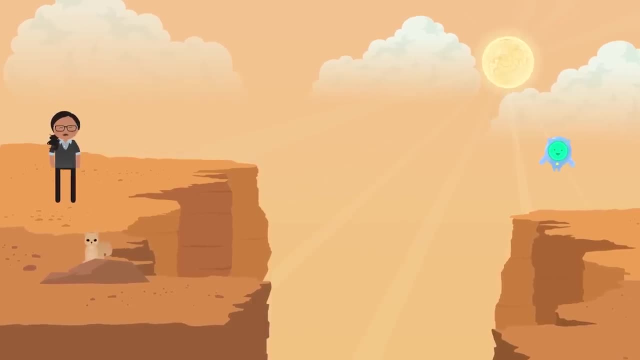 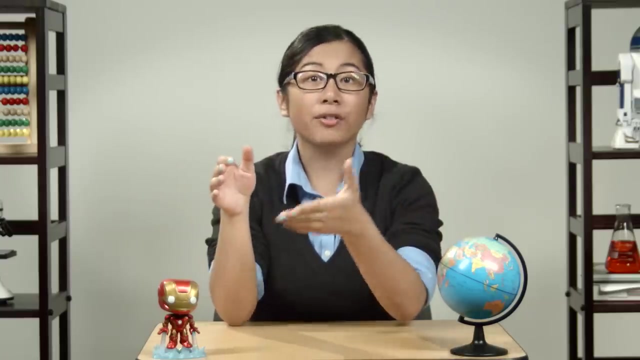 Pretend you're on one side of a very big canyon and you need to get to the other side. So that's the problem you need to solve, right: How to cross this very big canyon, Sort of, but not exactly. We can do better. 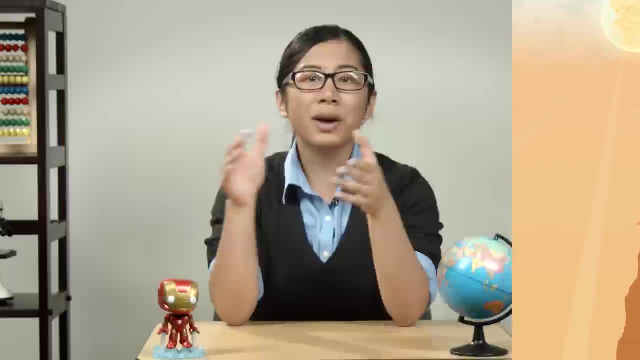 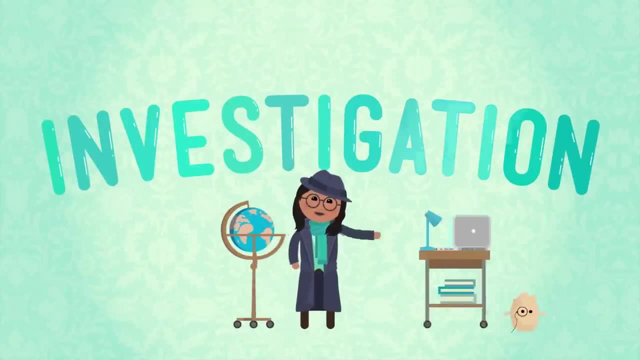 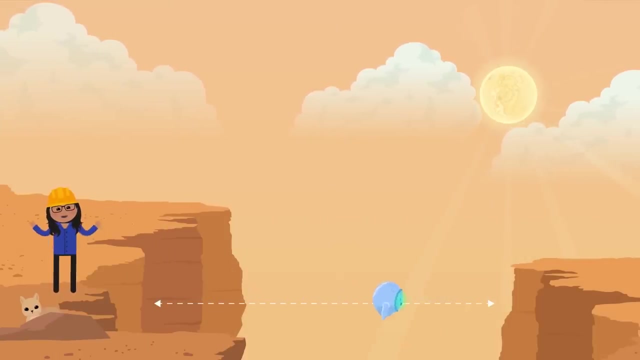 If I was an engineer and found myself on one side of that huge canyon, here's how I'd go about identifying the problem. I'd ask questions, a lot of questions, all the questions. Hmm, I need to cross this very big canyon, but is that my actual problem? Hmm, this canyon is. 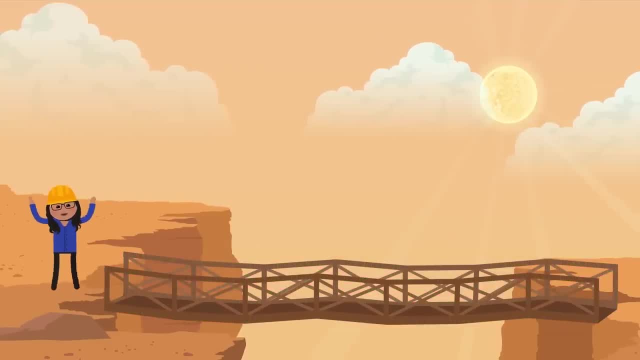 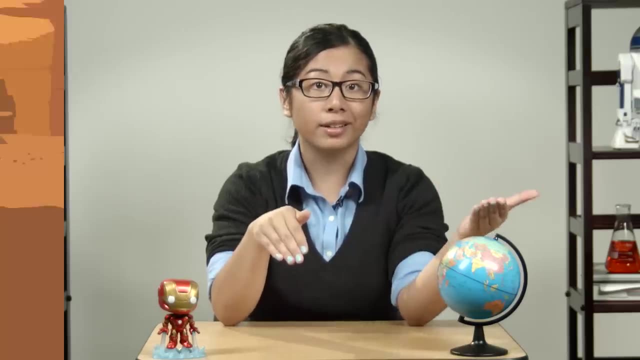 very big and I need to get to the other side. I know I'll cross a bridge. Wait, is there a bridge? Uh, yeah, there's no bridge. Okay, can I climb down one side of the canyon and then up the other side? 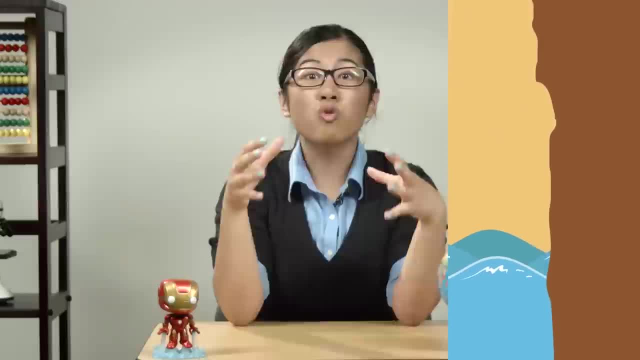 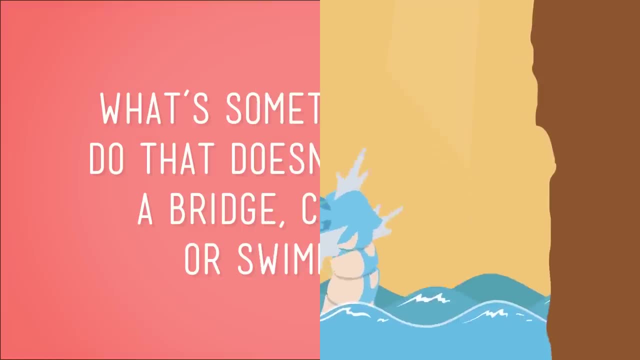 Uh, definitely not Way too deep. Plus, there's a roaring river at the bottom I'd have to figure out how to cross. So I can't cross the canyon by bridge, I can't climb down and up and I can't swim across it. 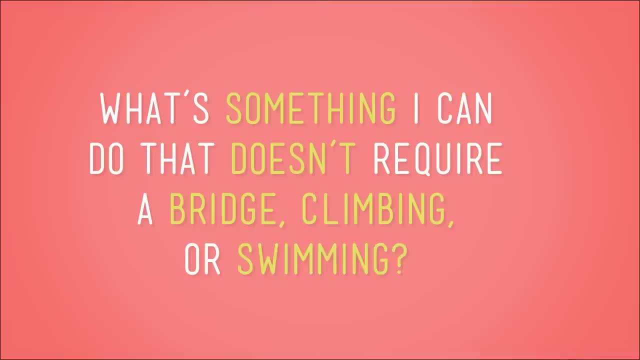 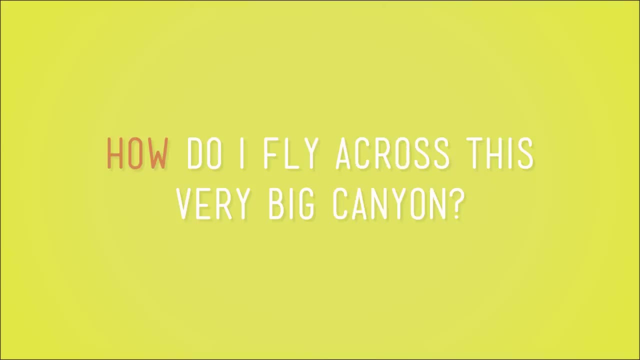 What's something I can do that doesn't require a bridge, climbing or swimming. I know I need to find a way to fly across the canyon, And that's my problem. More importantly, that's my solvable problem: How do I fly across this very big canyon? 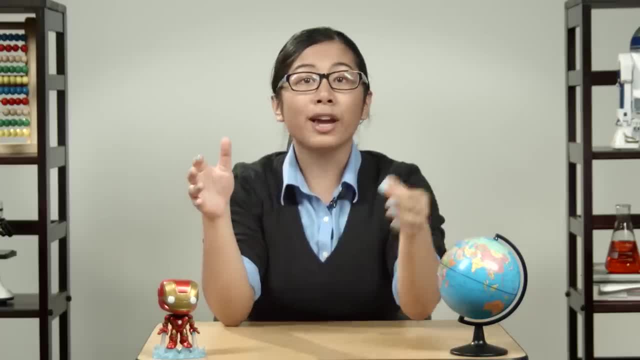 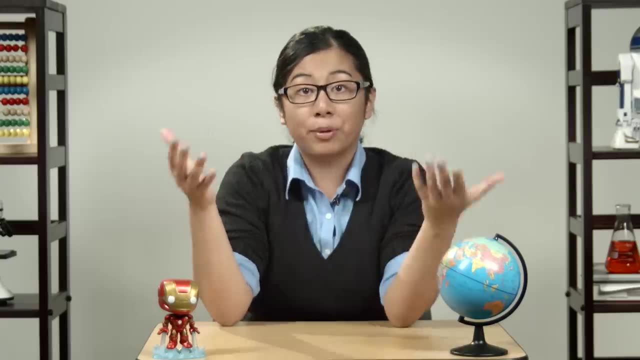 It took a little bit of thinking and a whole lot of questions. But how can you fly across the canyon is an easier problem to address than the much less specific. I'm on one side of a big canyon and I want to get to the other side and I don't know how to get across it. 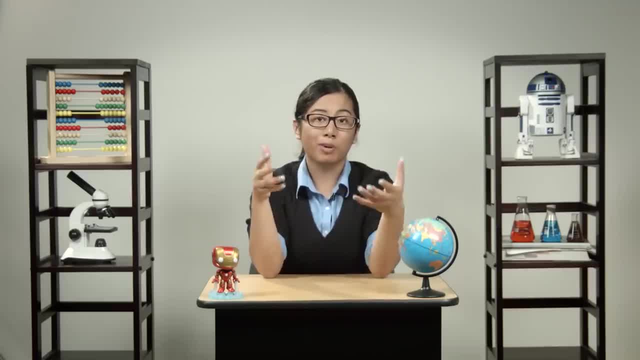 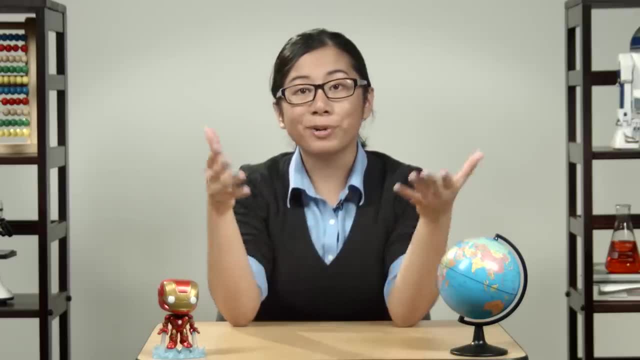 Which, strictly speaking, isn't a question. It's just complaining about a problem really loudly. So defining the problem in a solvable way is really key to being a good engineer. While that first step might seem pretty easy, make sure you treat it like the super important step that it is. 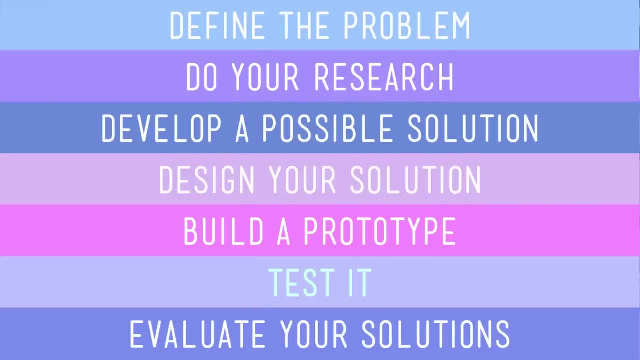 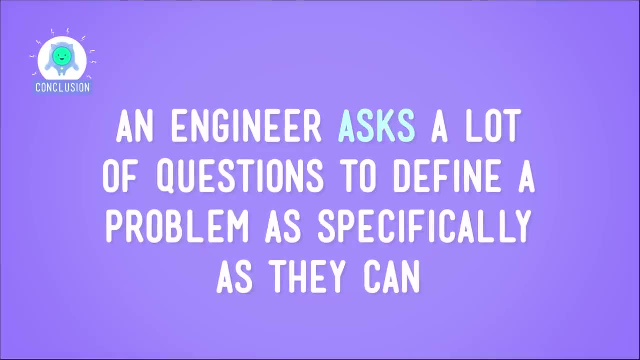 Because it sets the stage for all of the steps of the engineering process that follow. If you don't define a potentially solvable problem from the start, you might never well solve it. So an engineer asks a lot of questions to define a problem as specifically as they can. 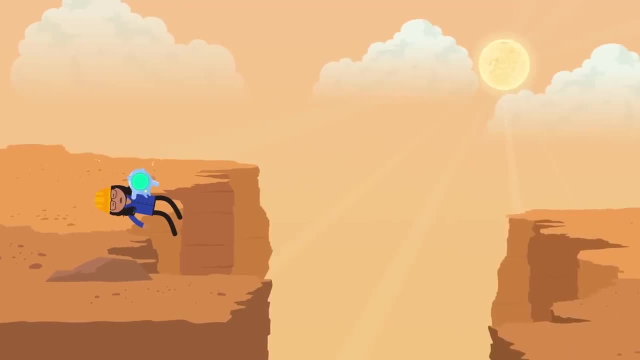 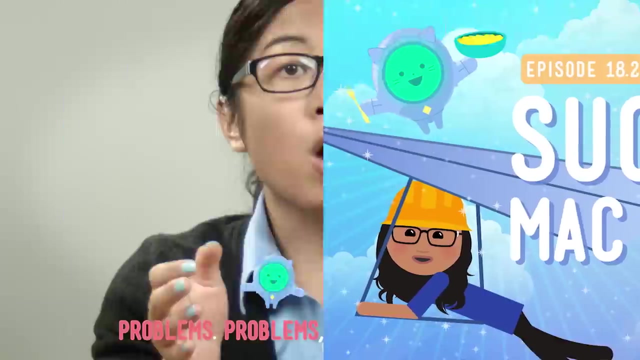 and most importantly, as something that can be solved. So how is engineer Sabrina going to find a way to fly across that gorge? You're going to have to solve that problem by watching our next lesson: Problems, problems, problems. We've been learning a lot about engineering lately. 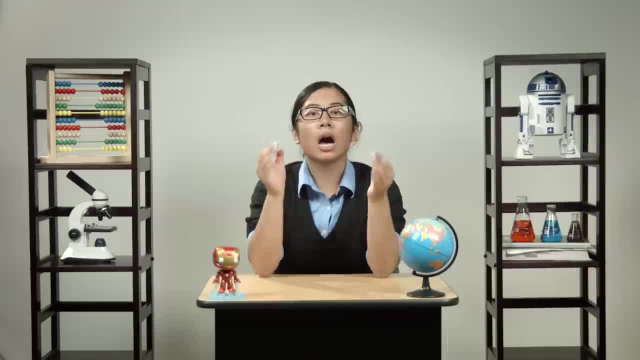 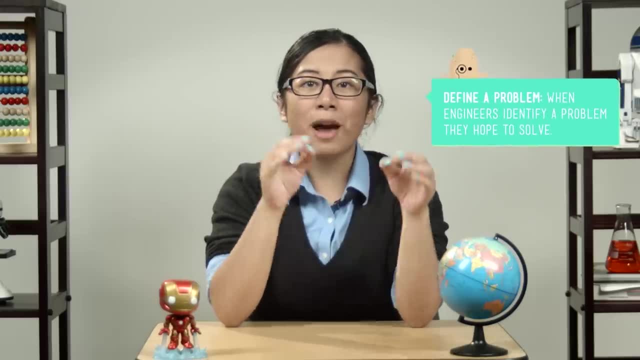 and engineering always starts with a problem that needs to be solved. But I'm tired of talking about problems, so let's talk about solutions instead. We've already learned about how engineers define problems. Now it's time to discover how they define success. 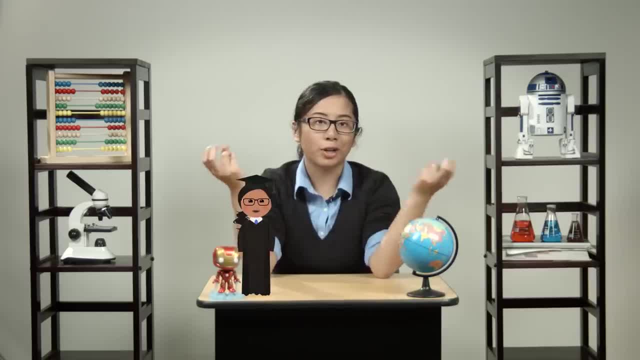 I don't mean how they define success, like in general, Like success is graduating from a good school, or success is getting a good bonus check at work, or success is winning a lifetime supply of macaroni and cheese- Although, I'm not going to lie, that sounds like success to me. 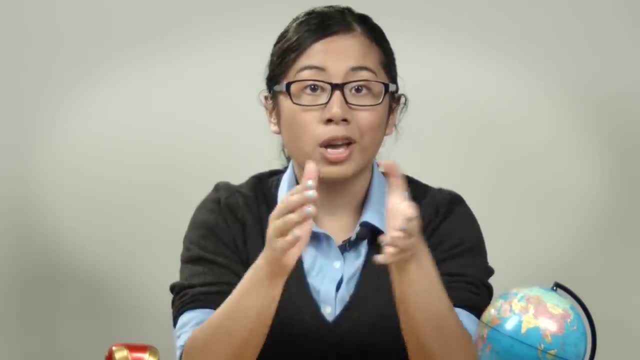 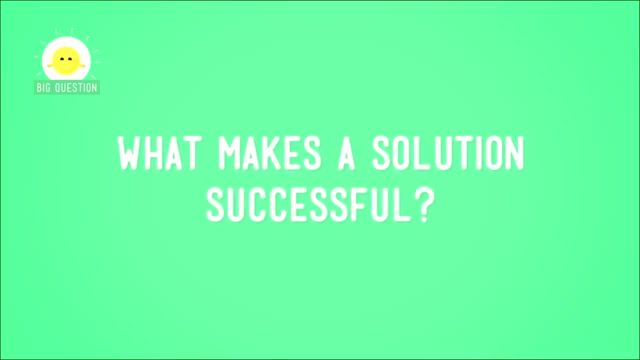 When engineers define success, they do it in relation to the problem they're trying to solve. So, for example, what does a successful solution to my problem look like? The big question we're asking today is: what makes a solution successful? Okay, let's back up a bit. 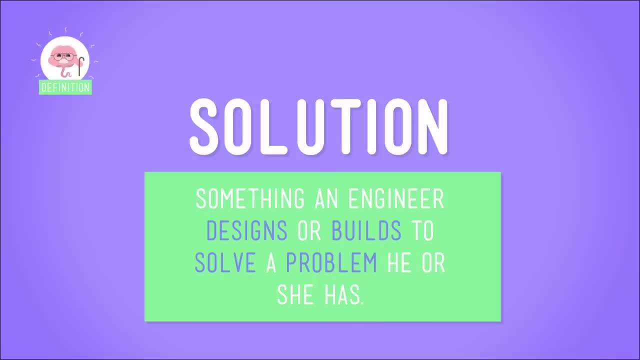 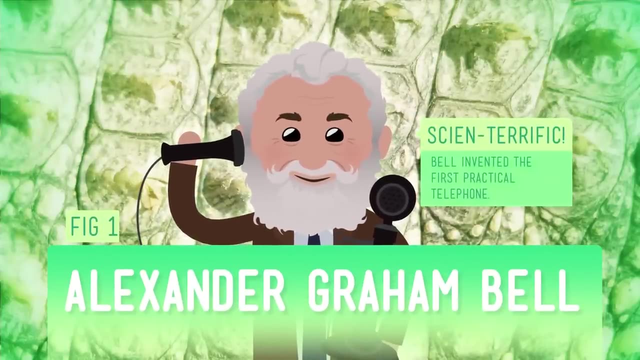 A solution is what again? A solution is something that an engineer designs or builds to solve a problem he or she has. Some solutions that engineers have come up with include the telephone, a solution to the problem of how people in different places can communicate with each other. 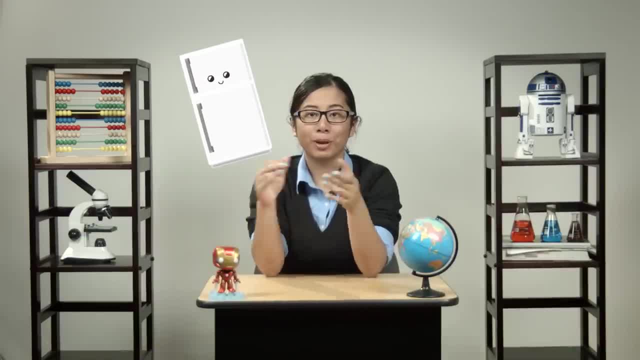 Or the refrigerator, a solution to not being able to keep food fresh for long periods of time, Or light bulbs, a solution to not being able to see at night, using something that's safer, brighter and more reliable than an open flame. 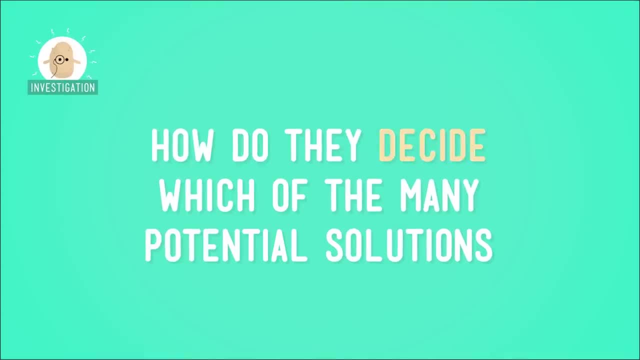 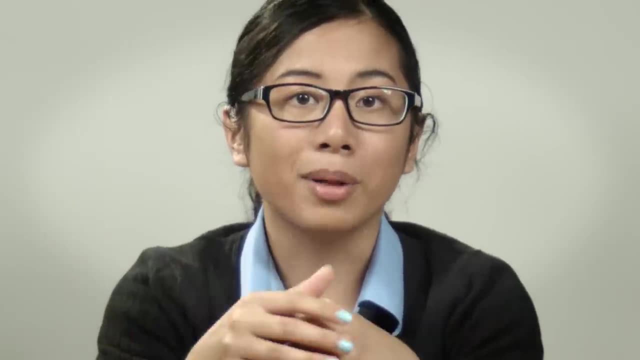 Every day, engineers design and build solutions, But how do they decide which of the many potential solutions that they brainstorm will be the most successful? I think an example would be helpful here, And we've already invented a fake problem, so why not invent a fake solution too? 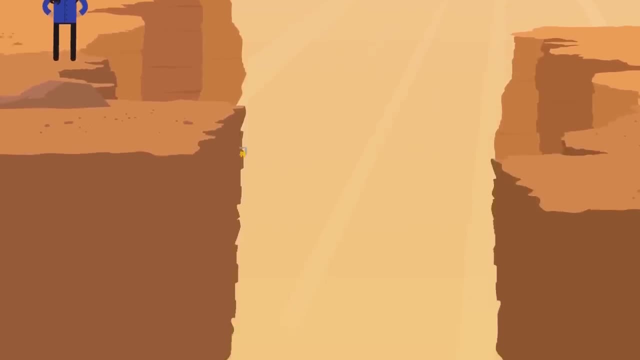 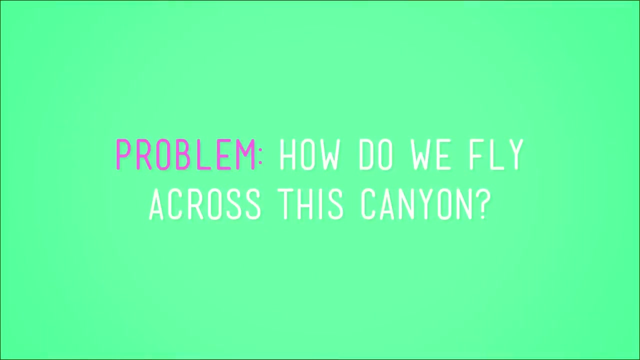 Back to the canyon, You know that insanely deep one with no bridge and the raging river at the bottom of it. Yeah, that one. The problem we defined at that spot was: how do we fly across this canyon? I'll be your stand-in engineer again. 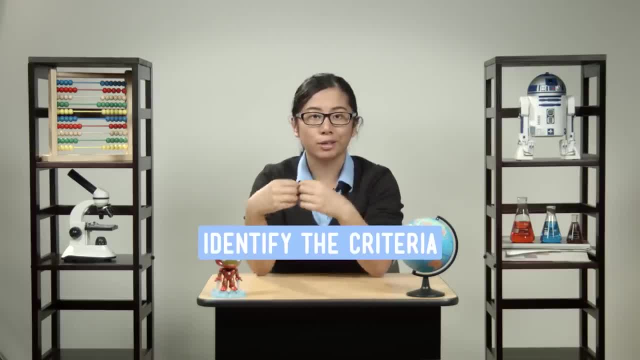 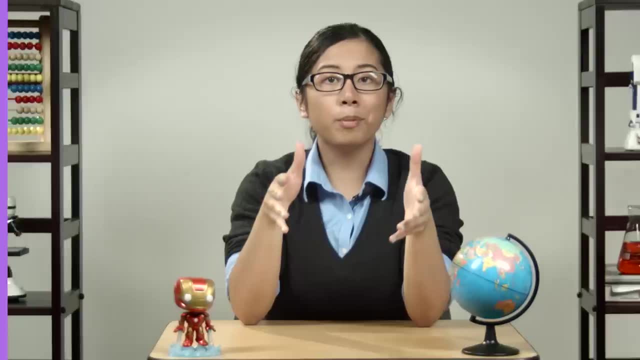 Being a good engineer, I know it's time to identify the criteria for my solution. Basically, I need to figure out what things my solution needs to do in order to be considered successful. Think of it like making a checklist Number one- it should get me to the other side. 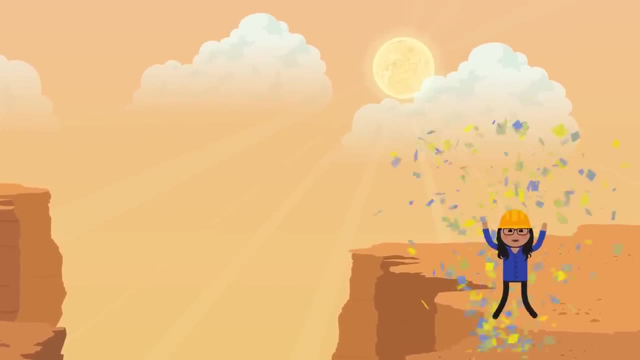 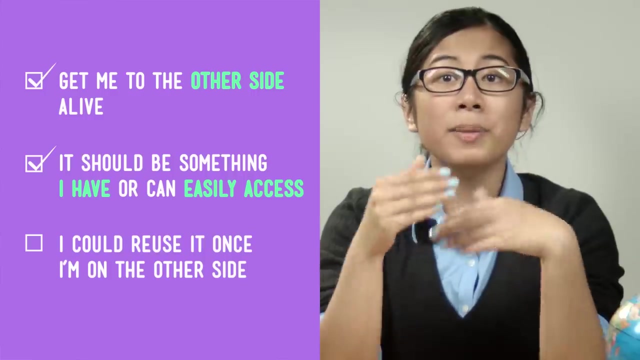 And let me be more specific: it should get me to the other side alive. Number two: it- the thing that gets me to the other side, should be something I currently have or can easily access. Number three: it would be nice if I could reuse whatever it is once I'm on the other side. 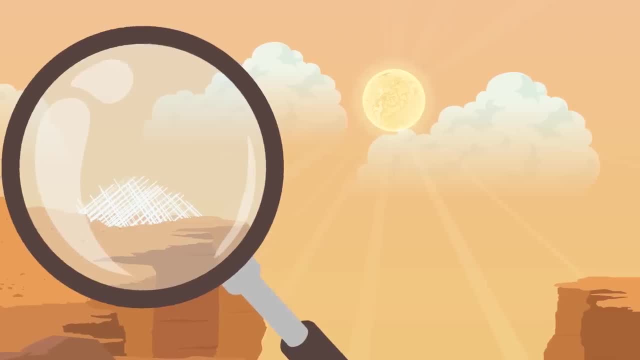 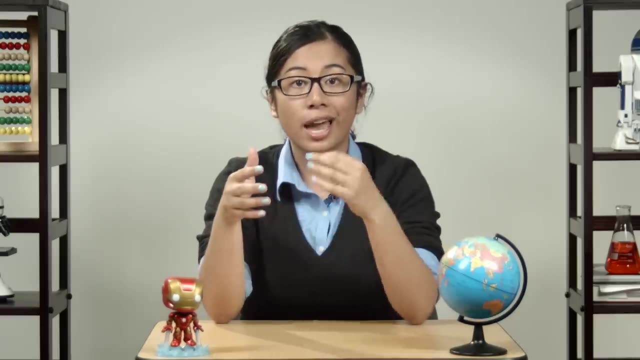 Now, if Superman's Fortress of Solitude was nearby, I'd snag him and make him fly me over this canyon, no prob, But sadly I don't have that. I won't have access to Superman's secret lair, So like any other engineer, I have to make do with what I have. 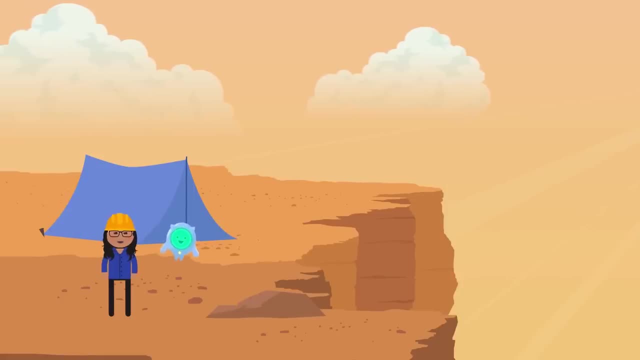 So what do I have? I've got the tent that I camped with and that's about it. You guys, I can make a hang glider out of my tent. It's a resource I already have and if I build it properly, 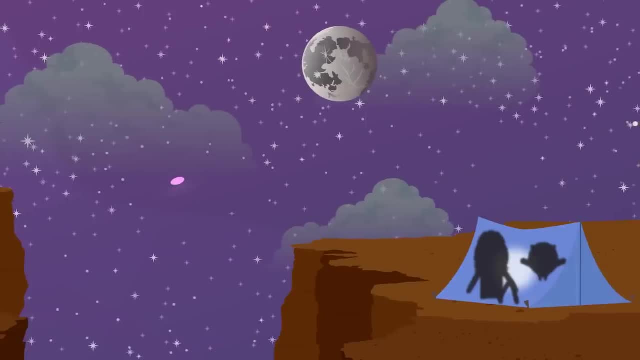 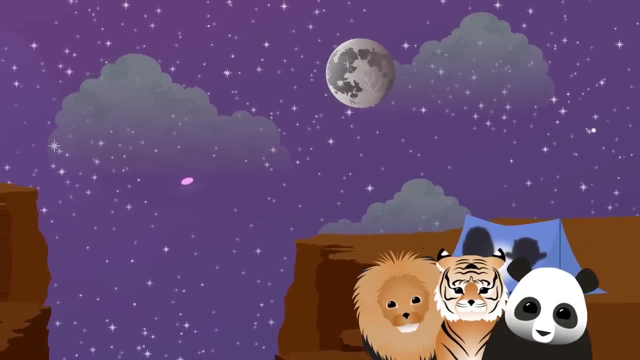 it will get me to the other side alive, which is ultimately where I want to be. Plus bonus, I can dismantle the glider on the other side and use the pieces for their original purpose: keeping me sheltered from lions and tigers and bears. 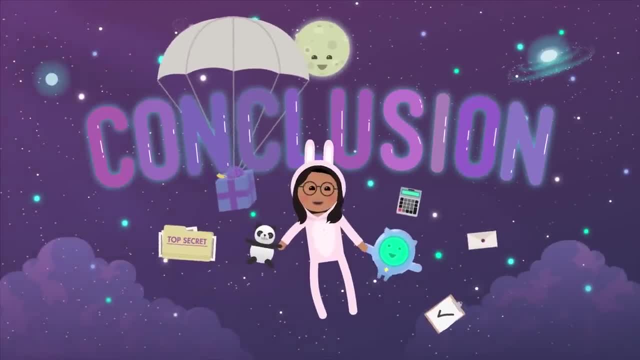 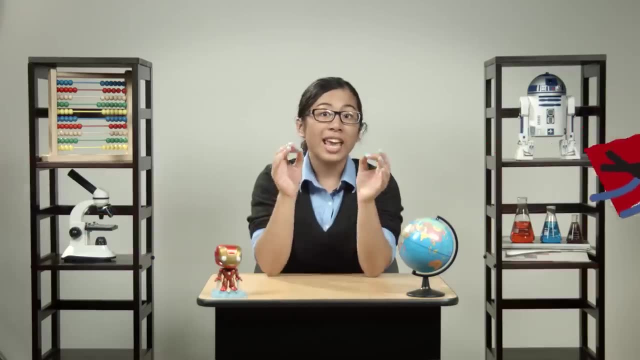 Oh my. So Superman's a solution in that if he were real and if I could somehow contact him to get him to carry me over this canyon, he could get me to the other side alive. But he's not the most successful solution because he doesn't meet all of my criteria. 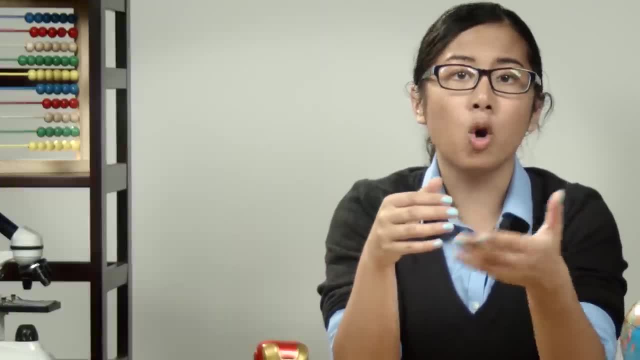 He's not currently with me and I can't easily find him. I mean, the whole point of a secret lair is that it's secret. So a hang glider meets all of my criteria, which means that's our solution. 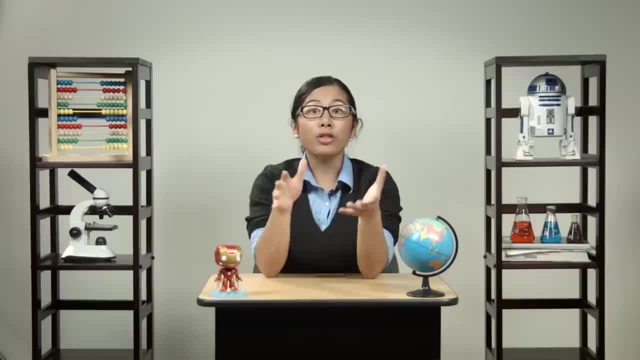 We'll fly across this very big canyon with a hang glider, And of all the solutions that an engineer can brainstorm to whatever problem he or she has, the most successful solution is the hang glider. So Superman's a solution in that if he were real and if I could somehow contact him to get him to carry me over this canyon, he could get me to the other side alive. 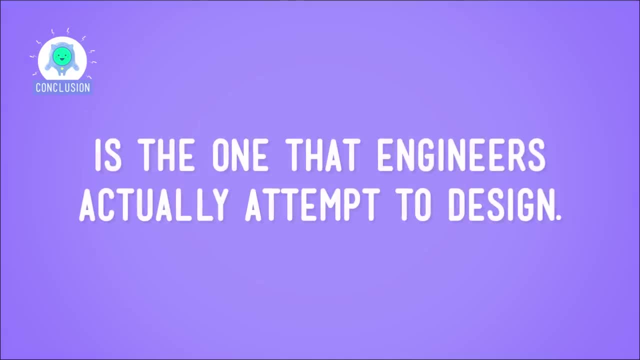 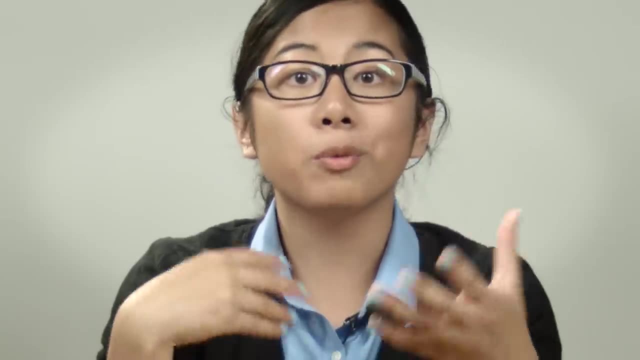 But the most successful one, the one that meets all of or most of the criteria, is the one that engineers actually attempt to design. Now, actually making a hang glider out of a tent is a different step in the engineering process, so it's one that we kind of- fortunately, don't have to mess with today. 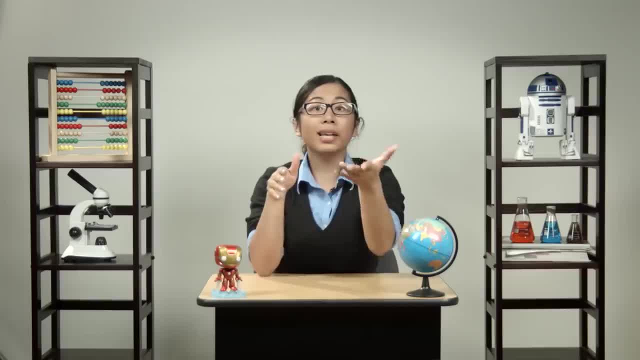 because I have zero idea about how to build or fly a hang glider. And anyway, remember that this is a totally fake, made-up solution. Don't go jumping into a canyon or anything with a tent, okay? We're here to solve problems, not create new ones. 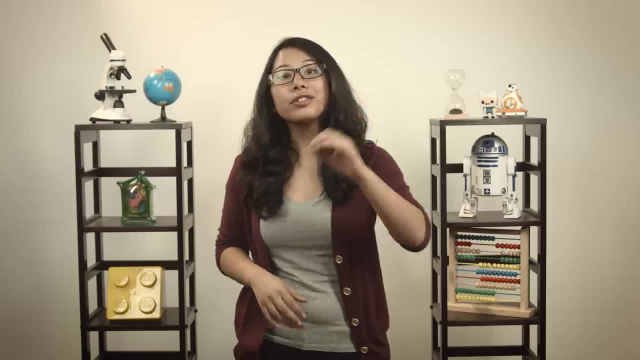 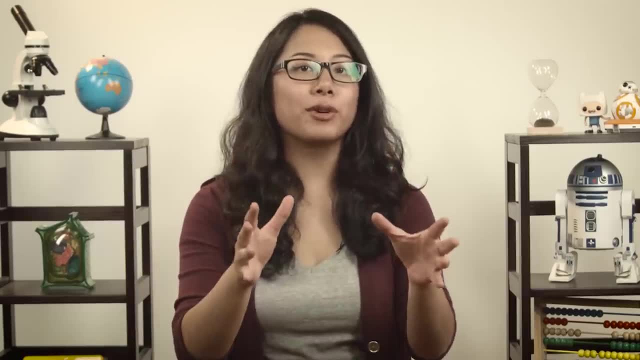 We've talked about problems And, hey, we've all got them, But there are other things we need to understand if we're going to be good engineers. One of the biggest concepts we need to tackle is variables. What can we change and what can't we change when testing our problems? 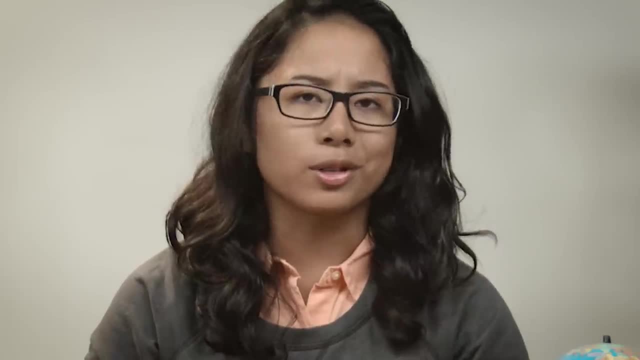 Everyone gets a case of the what-if. sometimes You know how you ask yourself questions like: what if I run out of popcorn and the movie's not over yet? Or what if it's raining when I walk home from school and I forgot my umbrella? 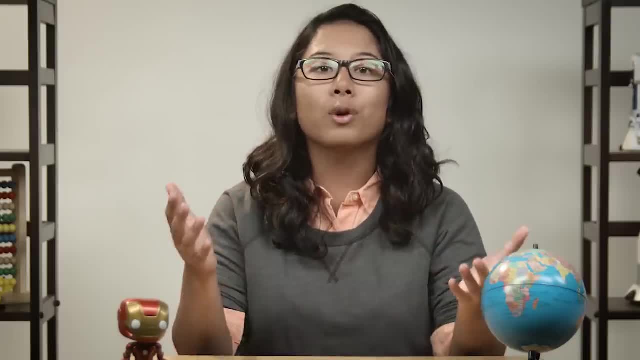 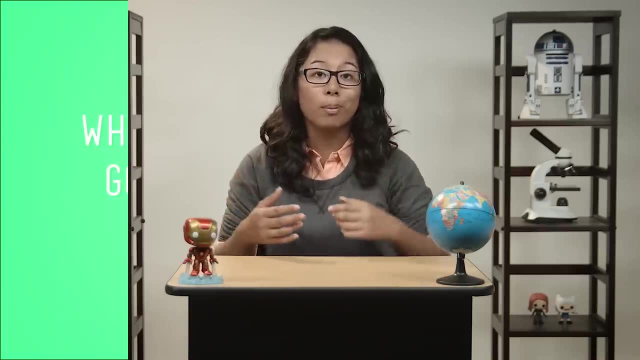 The threat is real people, But you know who asks themselves what-if questions every day. Engineers, These kinds of questions are really important when you're trying to come up with possible solutions to a problem Like what if we tried to cross a gorge by building a hang glider from a tent? 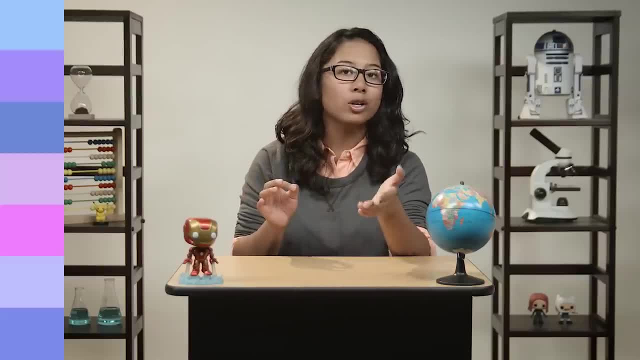 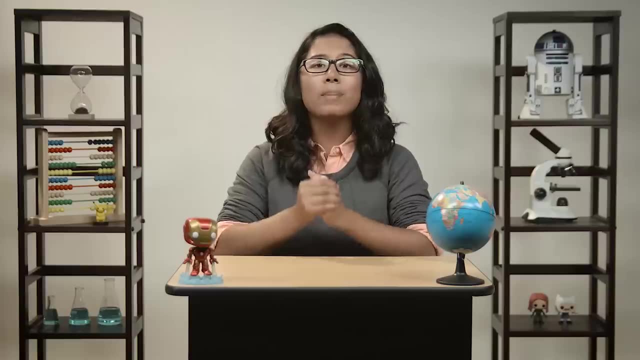 Remember that To come up with solutions to problems like crossing a gorge, you already know that engineers use a series of steps known as the trusty engineering process. A quick recap: We started by defining a solvable problem. In our case, how can we get across the gorge? 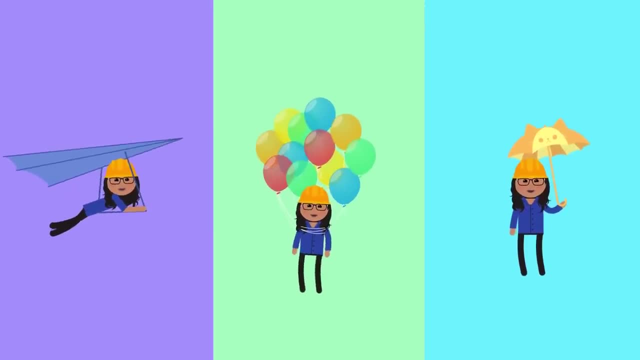 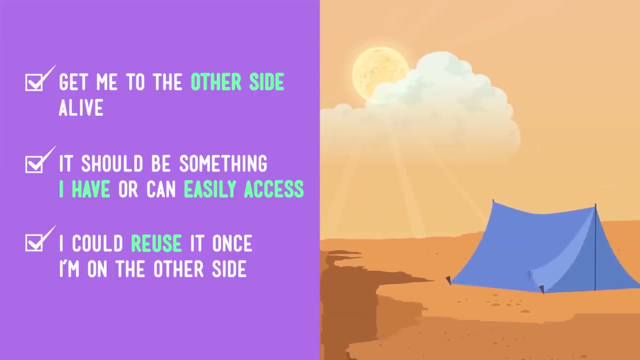 We looked at more than one solution and chose a solution that met our criteria. It used the materials we had available and it would successfully get us across the gorge in one piece. Plus, we could reuse the pieces afterward. Then, in the real world, an engineer would build a prototype of the solution. 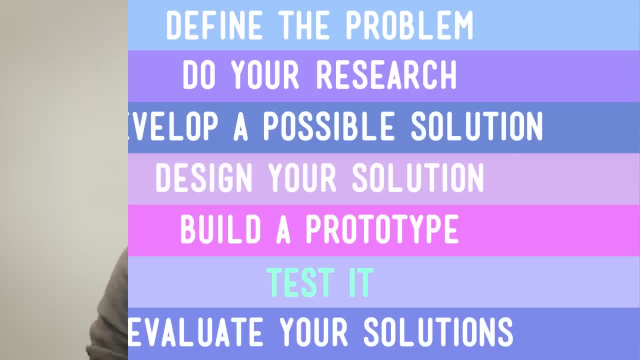 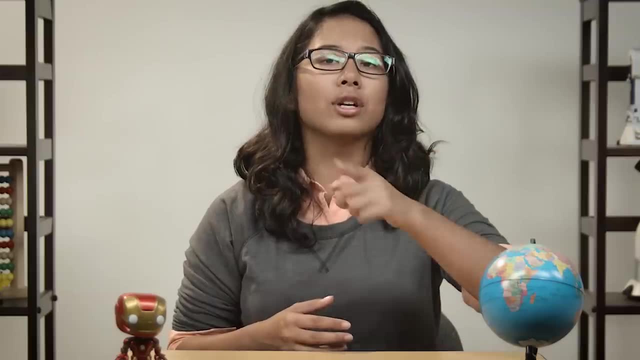 and test a bunch of prototypes before actually using it, And if the solution didn't work, they'd go back to the drawing board. Engineers are not quitters, And there's something else engineers do during the process that we haven't talked about yet. 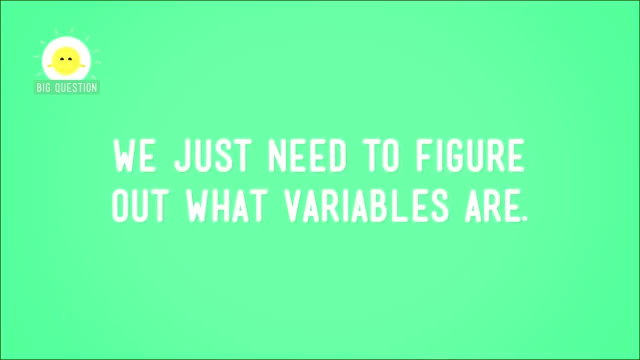 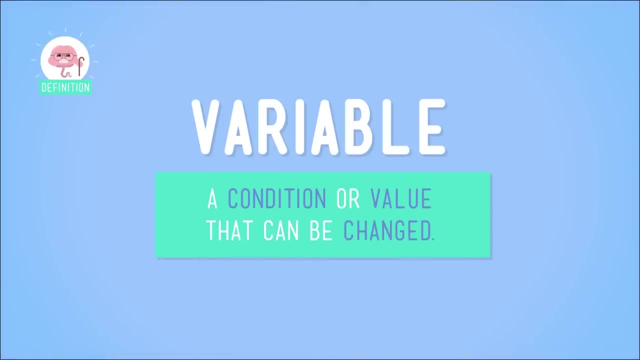 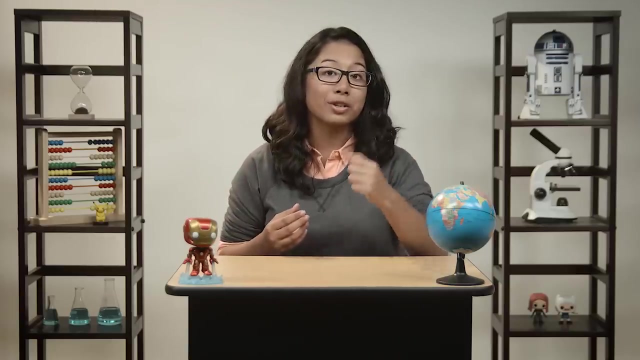 and that's defining variables, Excellent. So now we just need to figure out what variables are. A variable is just a condition or a value that can be changed, And sometimes a variable is something we can control, where we, as engineers, do the changing. 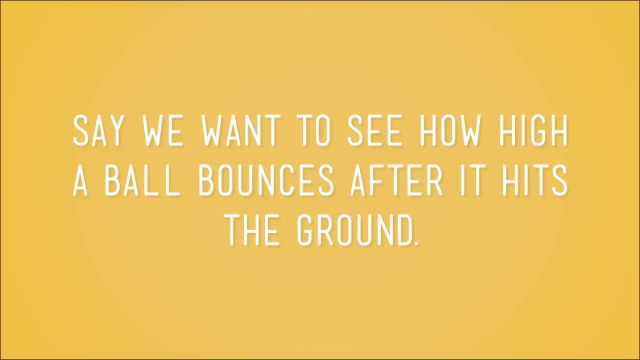 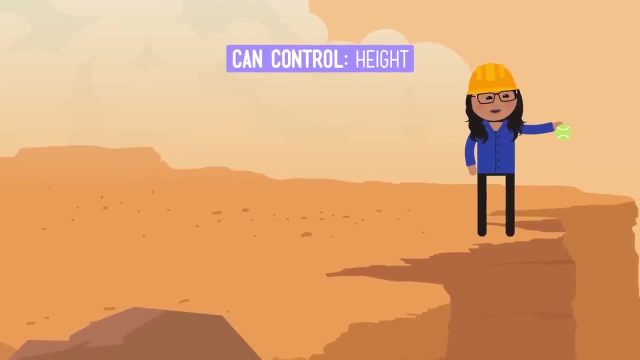 But other times variables are totally out of our control. So say, we want to see how high a ball bounces after it hits the ground. Let's identify some of the variables involved in that We can change the height from which we drop the ball. 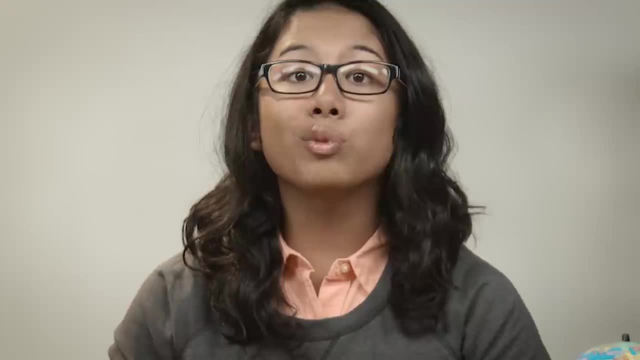 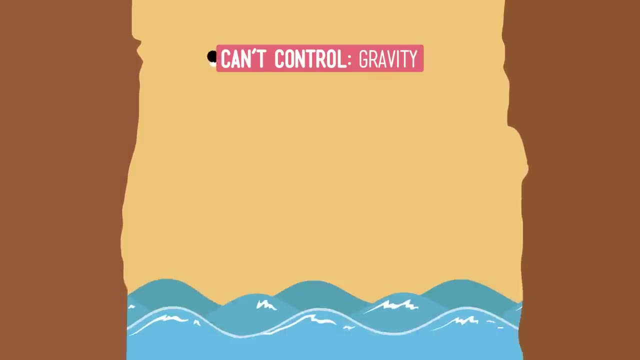 Or we can change the kind of ball we drop. Those are conditions we can change, But one thing we can't change is the gravity that pulls the ball down. So if we drop a ball towards the center of the earth after we drop it, that's not a variable we can control. 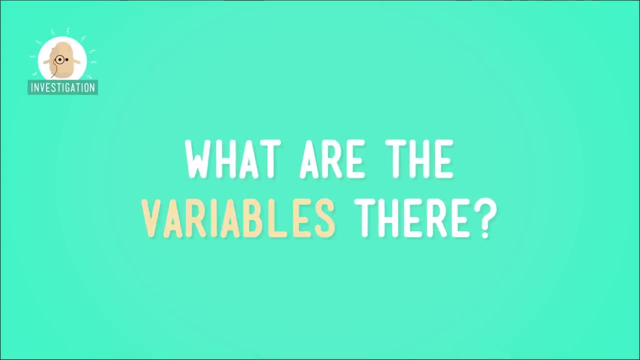 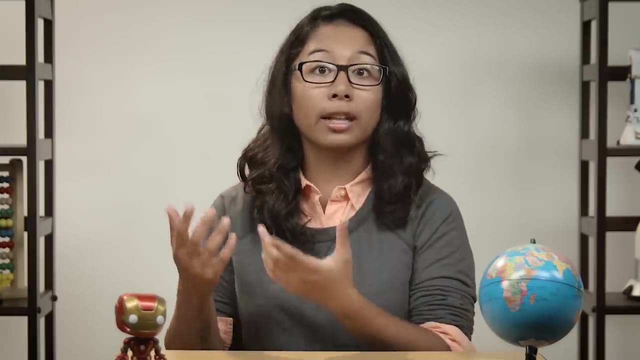 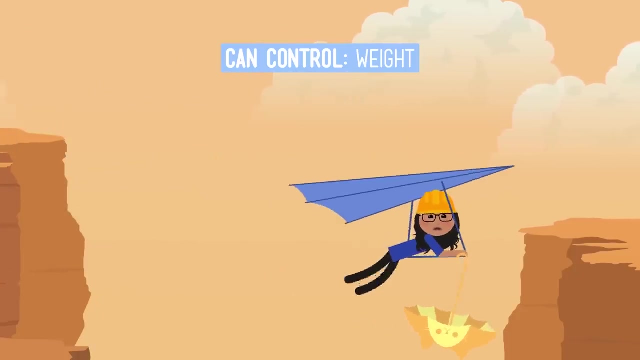 Now, what about our attempt to cross that giant gorge? What are the variables there? First, let's think about the variables that we can control. One variable we can change is the weight of our hang glider. We can reduce the weight that it has to carry by, say, leaving our umbrella behind. 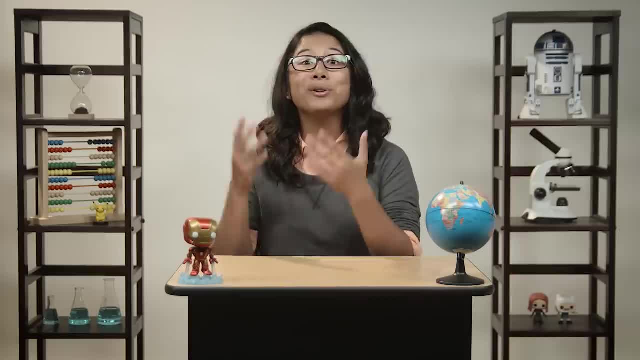 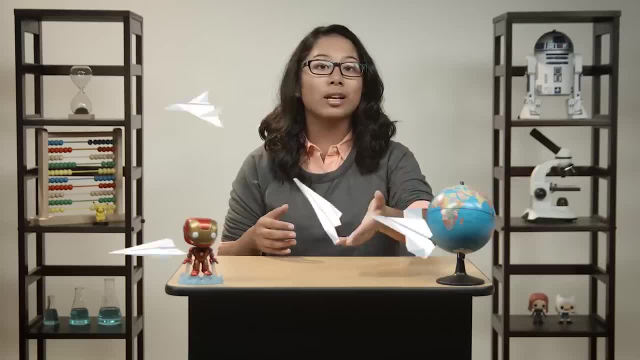 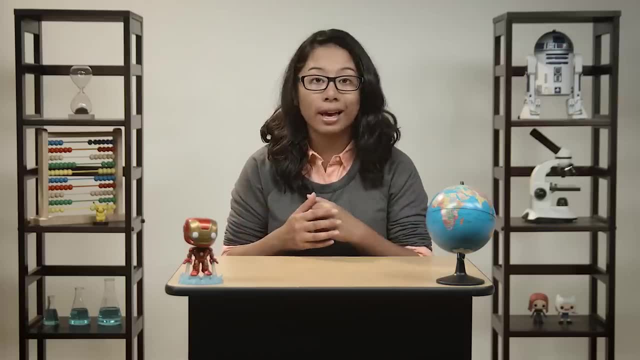 We can also change part of the hang glider's weight. If you've ever built a paper airplane, you know that you can change things like the size or the angle of the wings. These things affect how far or high the airplane flies. The same goes for our hang glider. 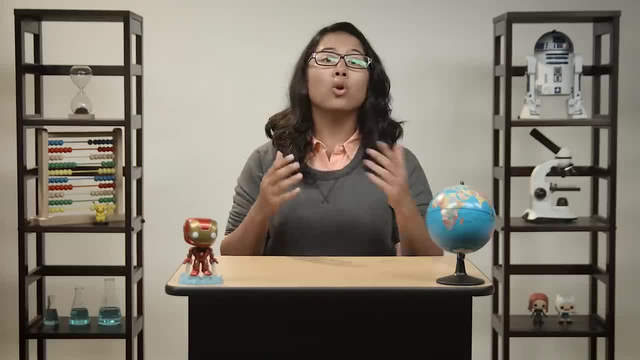 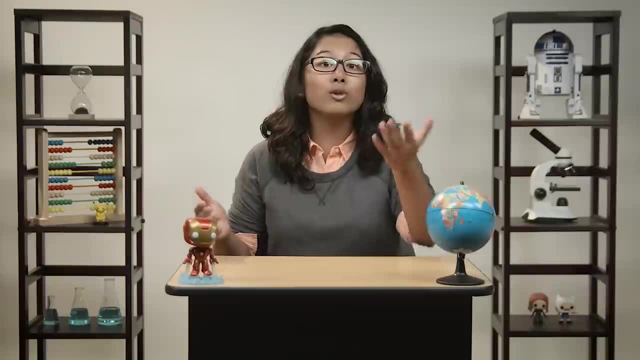 What about variables? we can't control. Let's talk wind. The wind over a gorge can be nice and breezy, It can also be forceful during a storm, But we can't control that. Sorry, Also, just like bouncing a ball, we can't control gravity. 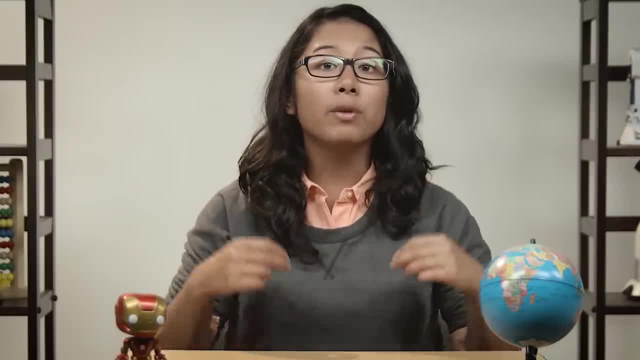 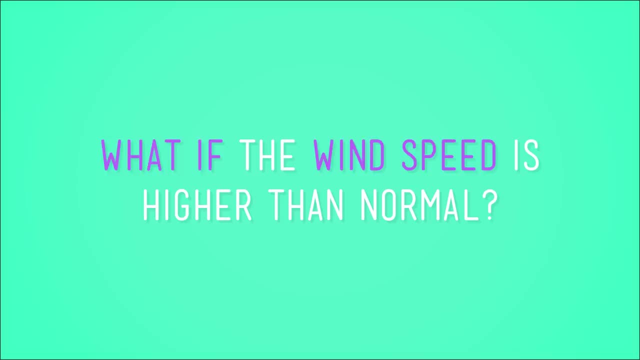 Now whether we can control the variables or not. once we've identified what could possibly change when we're trying to solve a problem, we can start asking what-if questions Like: what if the wind speed is higher than normal, Or what if we decide to leave our umbrella behind? 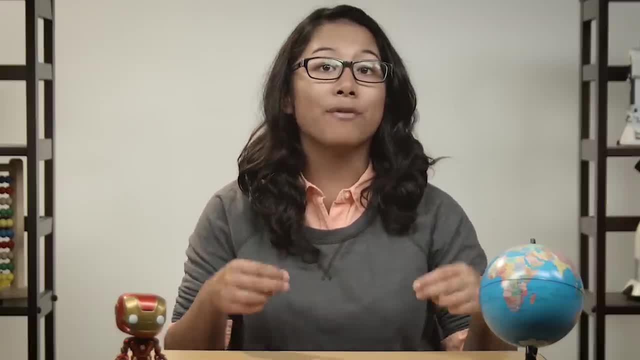 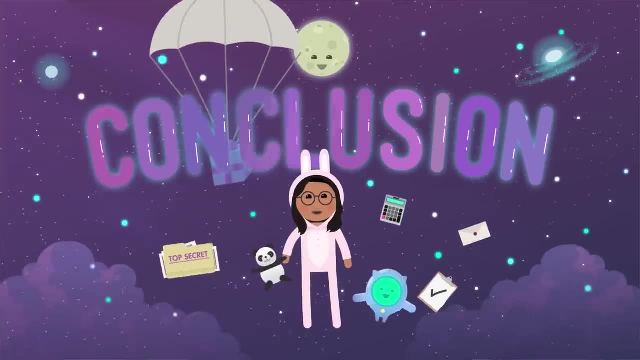 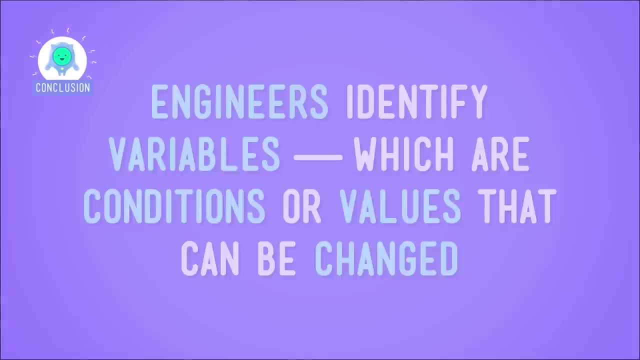 We can use the answers to those what-if questions to help us decide if our solution is going to work, Which would be nice to know before we go flying off into the gorge, right? So engineers identify variables, which are conditions or values that can be changed. 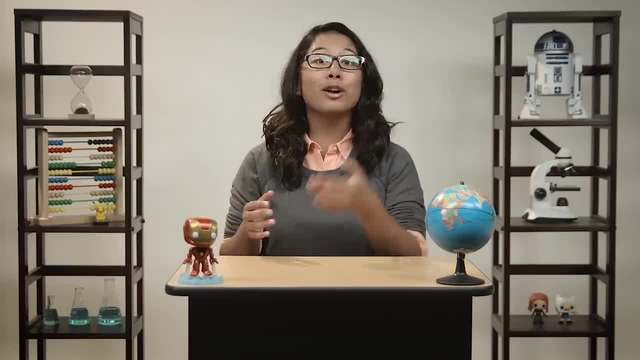 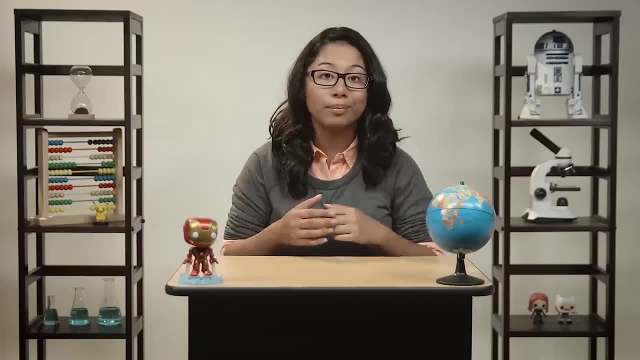 when they're looking at and testing solutions to a problem, And by asking yourself what-if questions you can practice your engineering skills. What-if questions can help you identify variables when looking at a problem. Just don't ever ask yourself what if I forget- something that I've learned in Sabrina's awesome engineering videos. 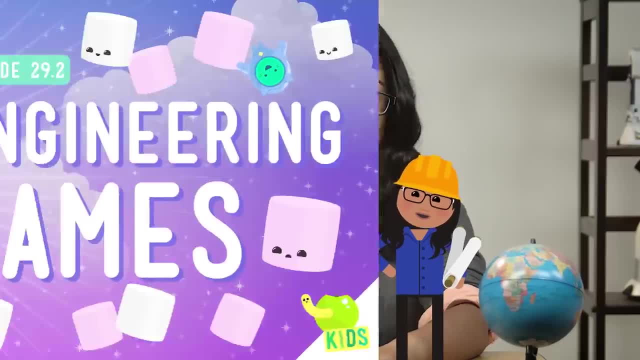 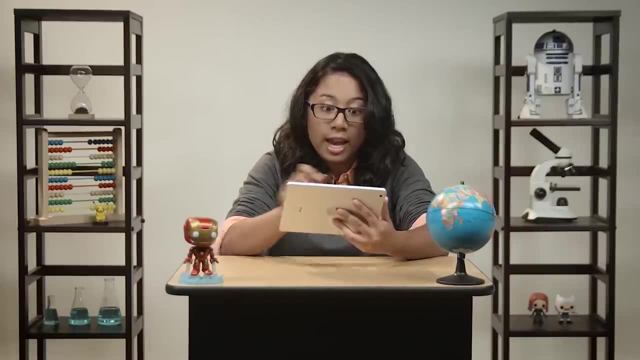 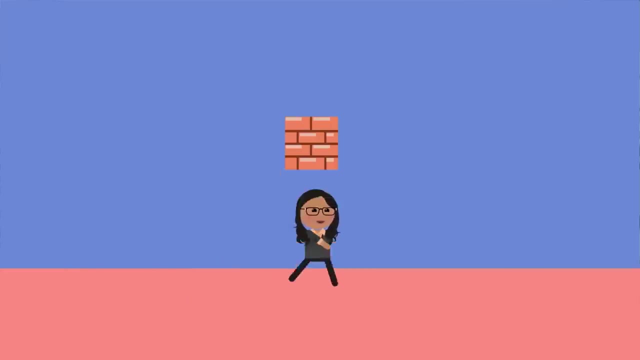 Because that's definitely not going to happen. Right, Catbot? Come on bird. And yes, Crushed it. I just beat a level that I've been stuck on for like a month. As any good gamer knows, it takes the right move to win. 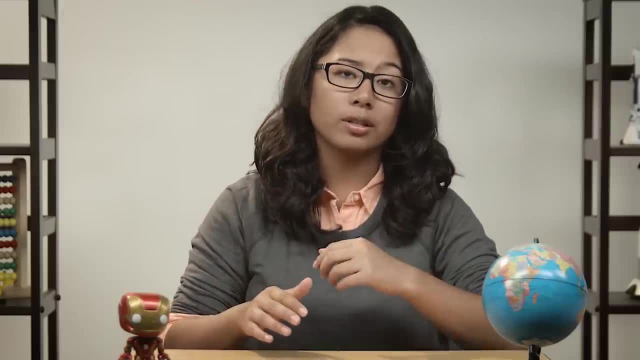 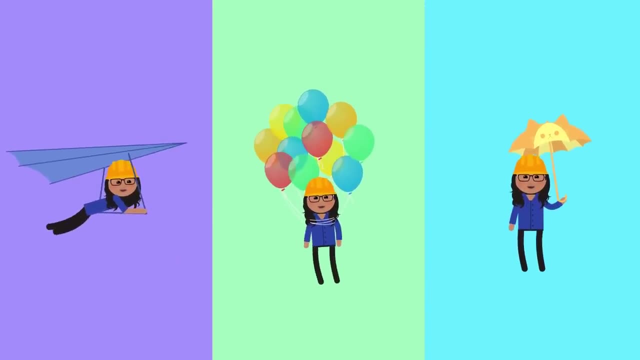 One wrong move and poof- A possible win can turn into a loss. The same thing is true for engineering. Last time we were thinking about the moves we could make that would guarantee the solution to our getting across the gorge problem was a success. 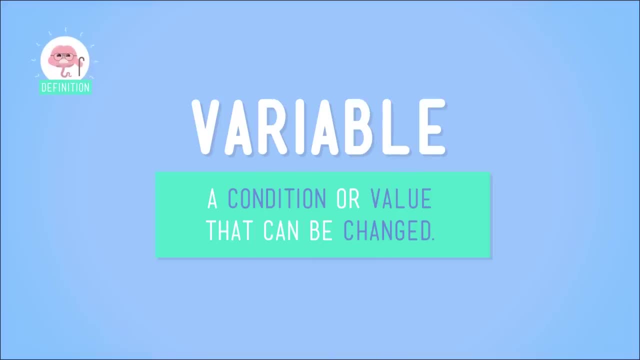 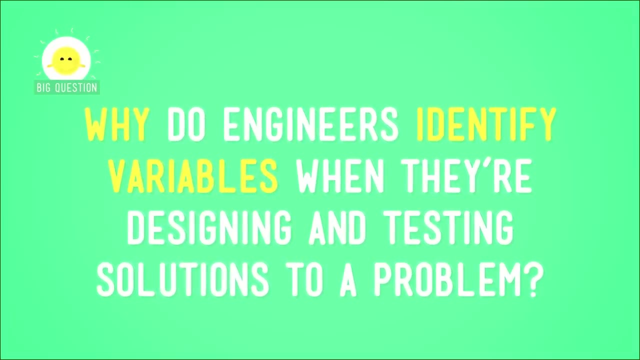 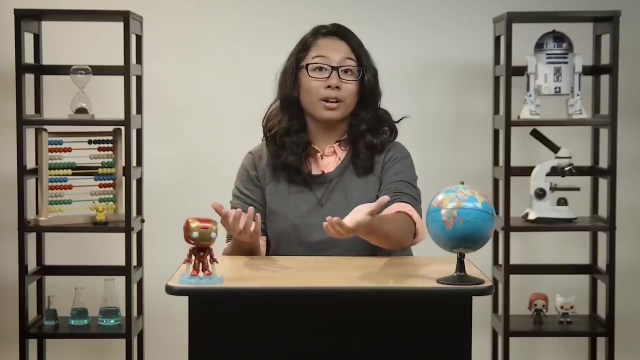 And that included identifying variables or the conditions or values involved in the problem. that can be changed. But what's the big deal? Why do engineers identify variables when they're designing and testing solutions to a problem? Remember, we can control some variables. 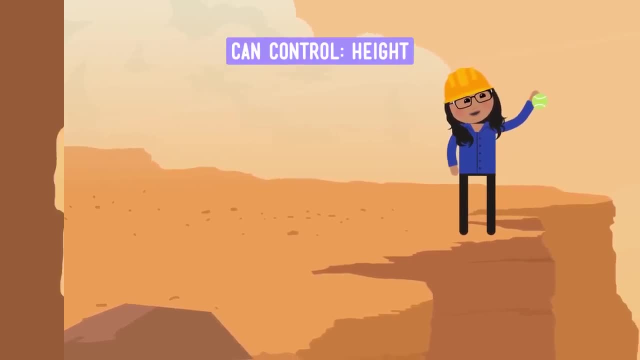 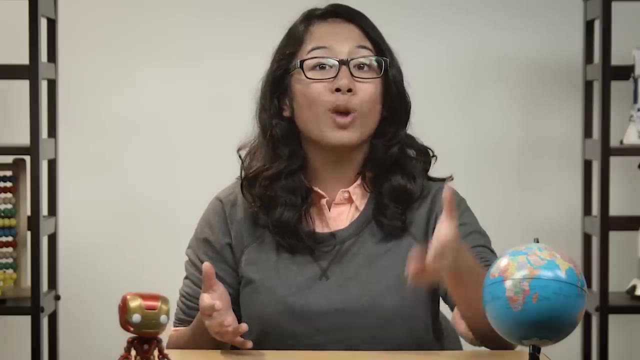 like the height from which we drop a ball to see how high it bounces. But there are variables we can't control, like gravity. Whether a solution to a problem turns out to be successful or not depends on picking the right way to change a variable. 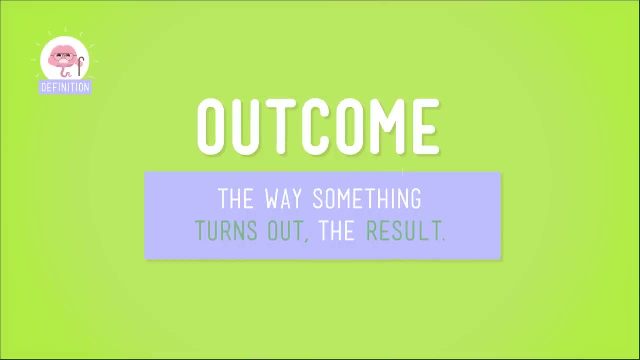 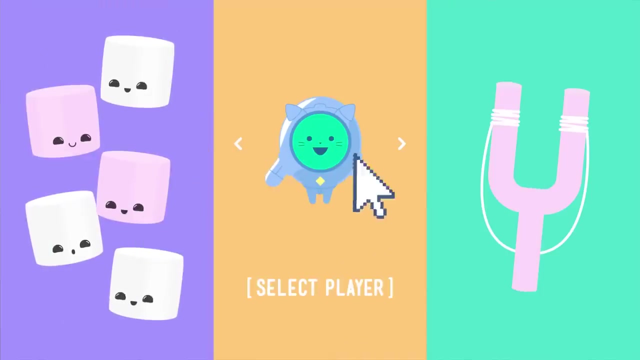 The way something turns out like, whether a solution solves the problem or not, is called an outcome. So let's see how changing variables can change an outcome by playing a game. The goal of this game is to knock down a pile of fluffy pink marshmallows. 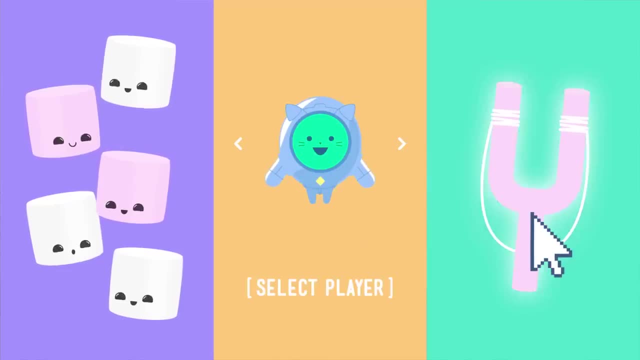 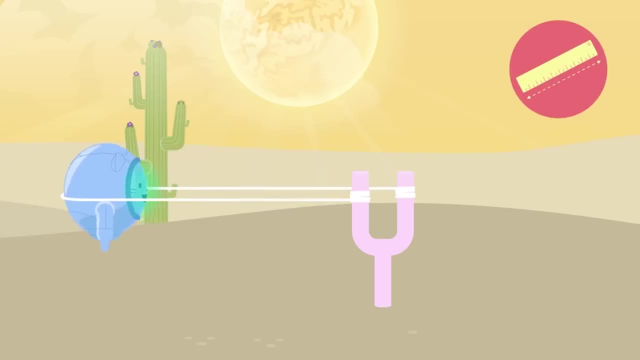 and to do that we launch Catbot into the pile using a slingshot. There are two variables here that we can control. We can change the angle of the launch and we can change how far we pull back on the slingshot. 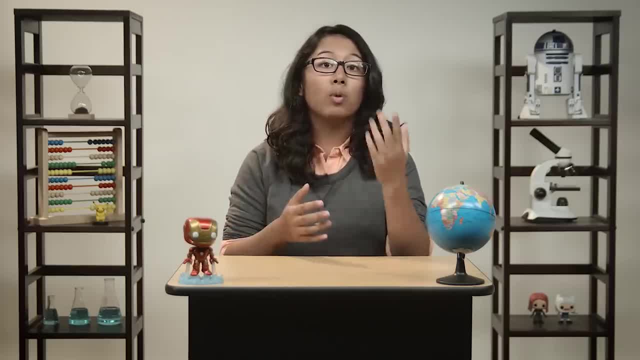 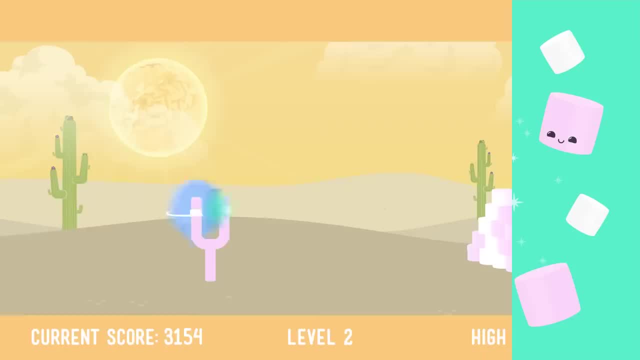 If we change either or both of these variables, then we can get one of three outcomes: We can knock over all of the fluffy marshmallows, knock over some of the fluffy marshmallows or miss the pile completely. Now I don't want to be stuck on this level for another month. 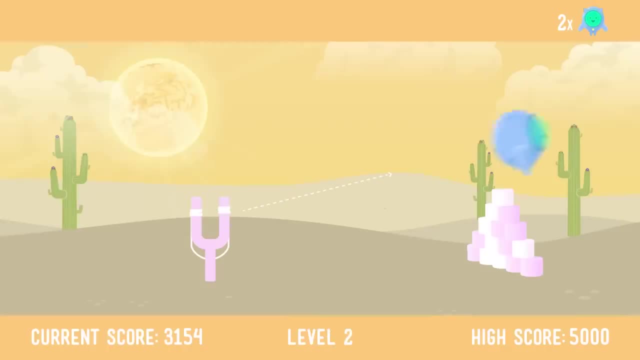 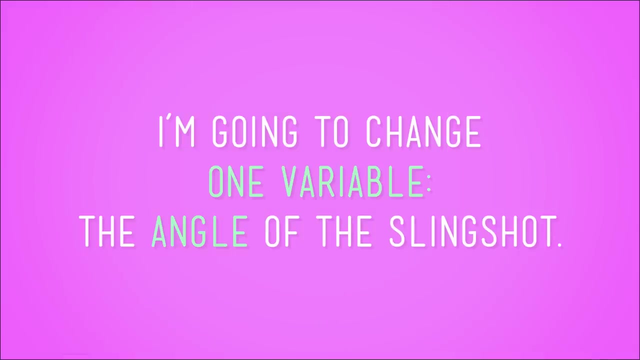 so I'm going for the complete knockdown outcome. Try number one And I miss Completely Boo. So I'm going to change one variable, the angle of the slingshot. But I want to pull back on the slingshot just as far as last time. 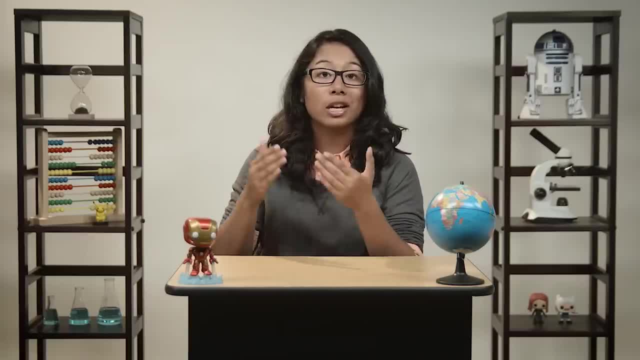 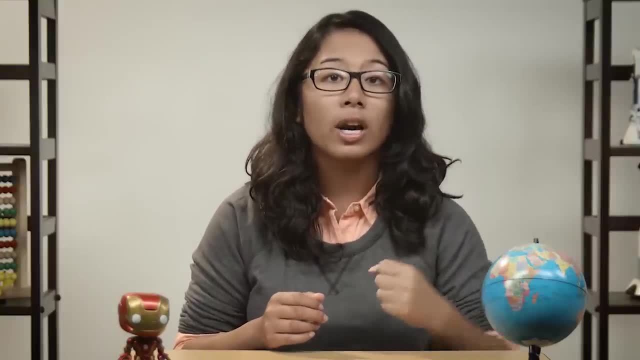 otherwise I won't be able to tell if the outcome of the second try is because I changed the angle or if I changed how hard I pulled. So let's see if changing the angle by pulling back just as hard as before gives me the outcome that I want. 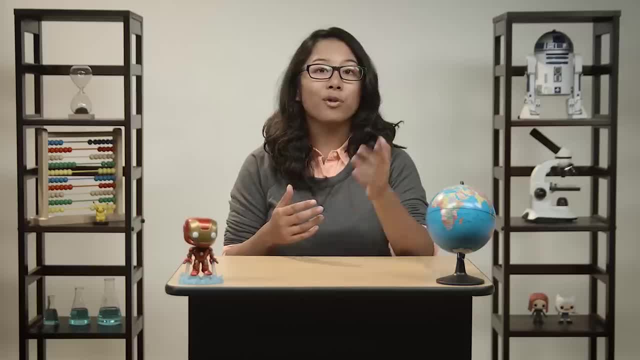 And score Total knockdown. Now, if I wanted to, for my second try I could have decided to change how hard I pulled on the slingshot. But if I did that, I'd have to keep the angle the same. 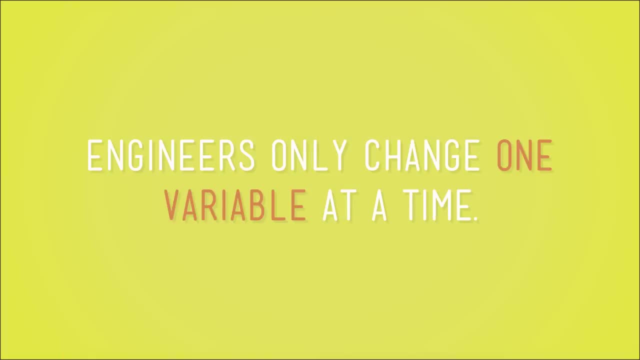 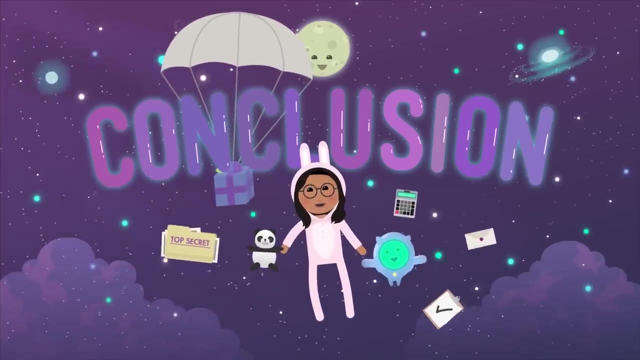 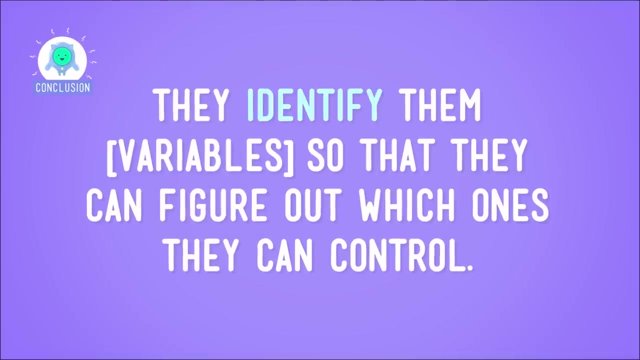 Bottom line engineers only change one variable at a time, Otherwise we can't tell why a solution works or doesn't work. So engineers don't just identify variables for fun, although it definitely can be. They identify them so they can figure out. 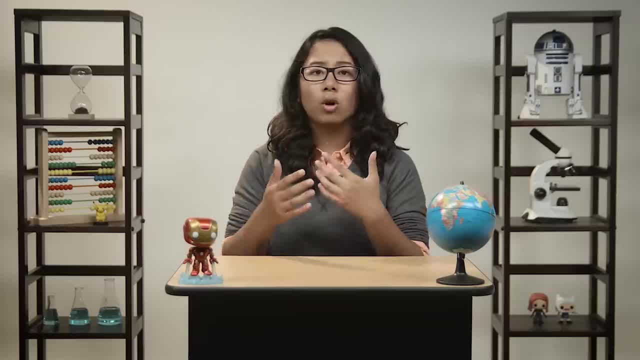 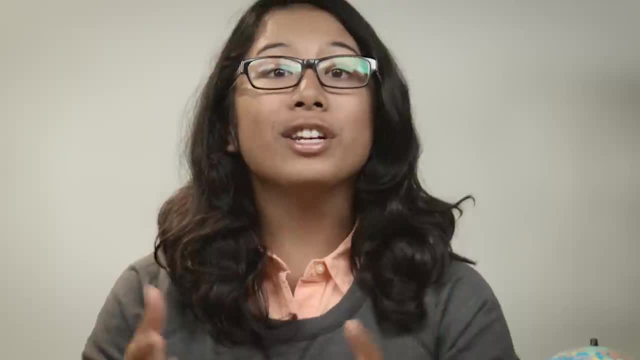 which ones they can control. That is, either change them or keep them the same, And that's important to know, because changing a variable can affect the outcome or result of a solution. So engineers change only one variable at a time when they test a solution. 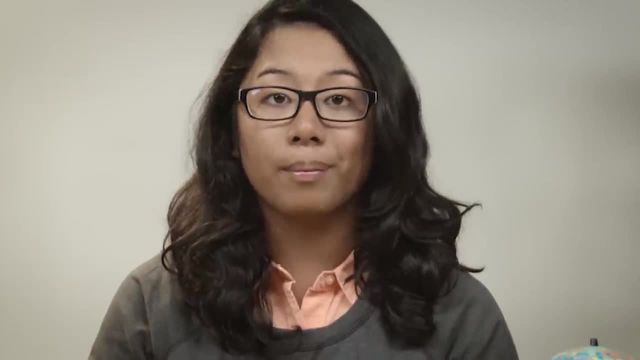 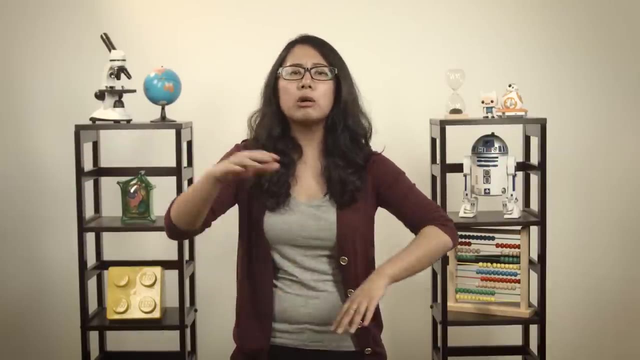 so they're sure of the connection between the variable and the outcome. Now it's back to my game. I'm coming for you: marshmallows, Problems, solutions, variables. There's a lot going on with engineering, But that makes sense. 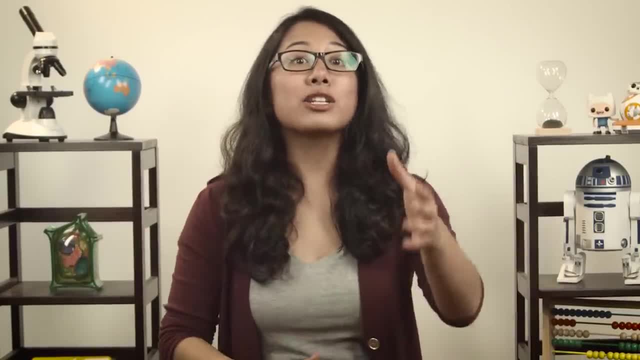 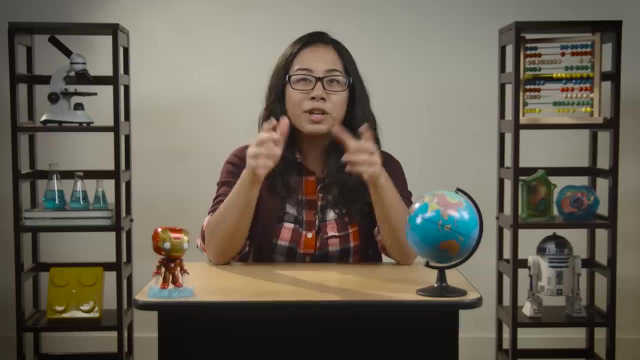 Engineers want things to work properly, especially when those things are robots, And that's why we're talking about robots and houses. Okay, listen up people, I need your help. You're going to have to help me engineer my way out of a challenge. 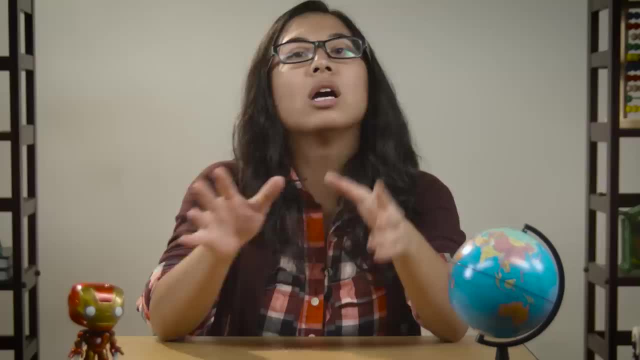 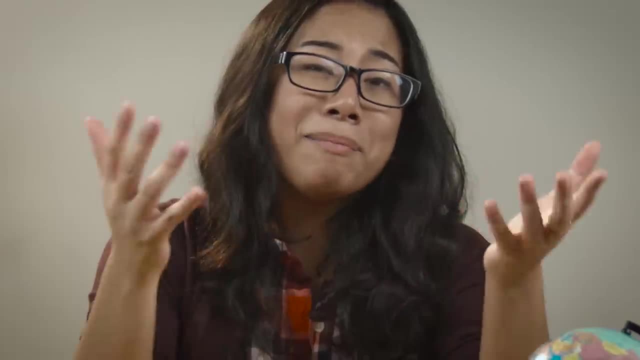 The challenge being I kind of dropped my phone down a sewer, I know, I know I was walking down the street and it slipped out of my hands and went right into the storm drain And, um, I kind of like it back. 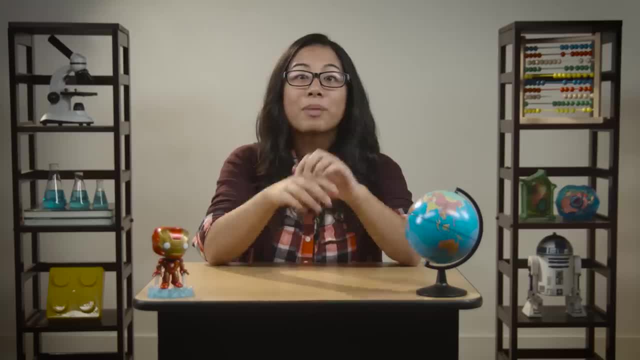 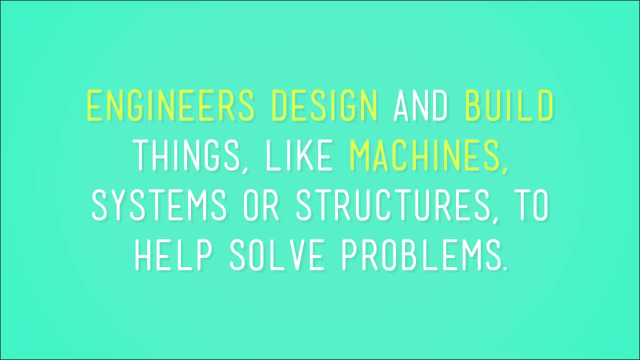 But that's where you come in, because this is exactly the kind of problem that can be solved with the help of engineering. You know that engineers design and build things like machines, systems or structures to help solve problems, And all kinds of problems, not just phones and sewers. 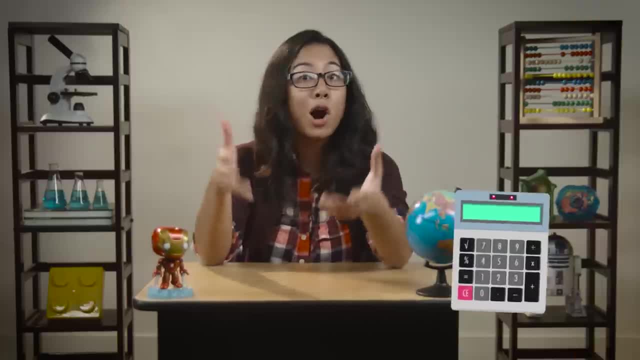 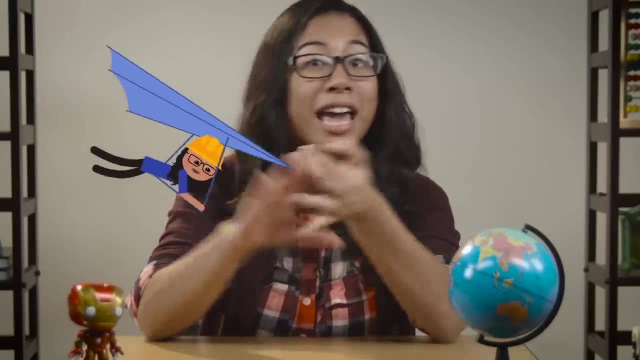 How can we cross deep, dangerous canyons? How can we solve complicated math problems if we don't have a pencil and paper? You can think an engineer for solutions to all of those problems, Hang gliders, calculators, and the list goes on and on. 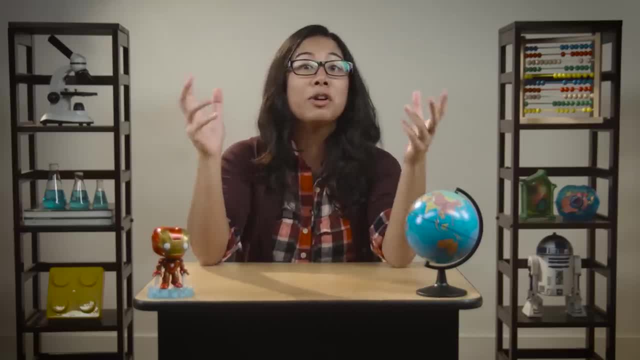 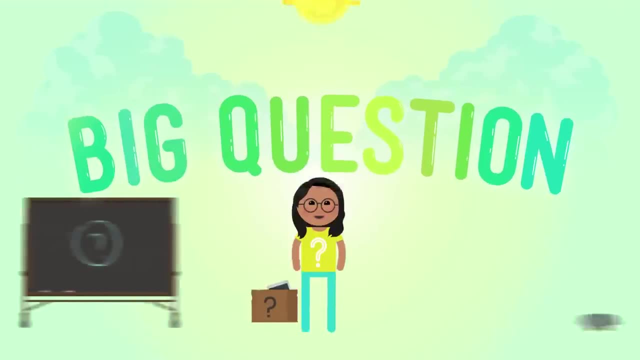 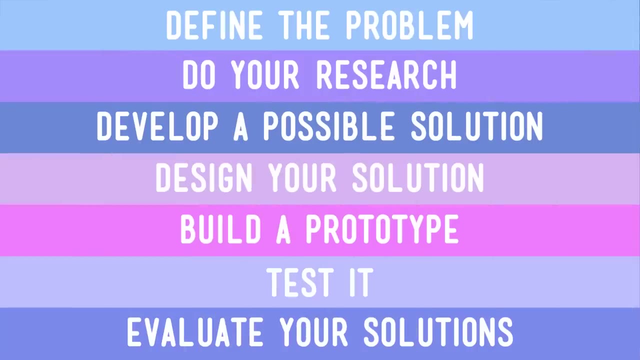 So now I need your help to unleash the power of engineering to fix my problem. So how do we use the engineering process to get my phone back? First, let's review the process. This is crucial. One define the problem. Okay, I need a way to retrieve my phone from a storm drain. 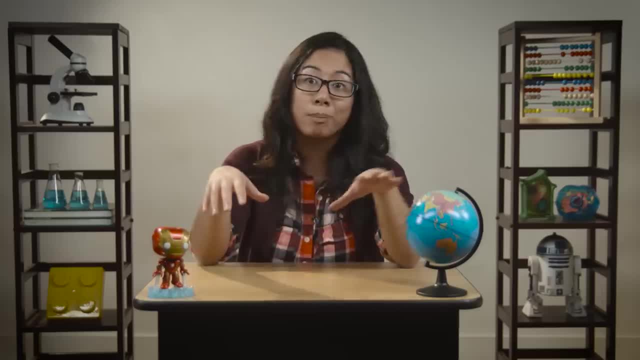 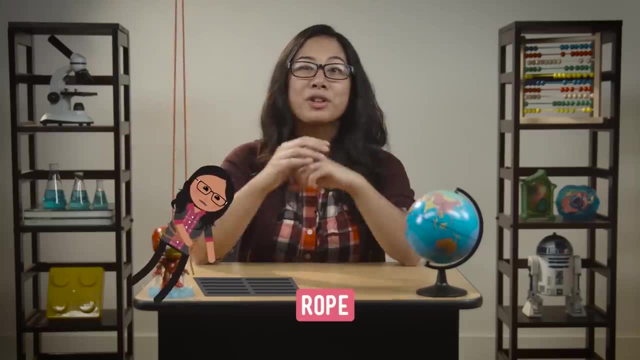 Two: consider solutions. There's more than one solution to any problem, so we need to think through different options and choose the best one. Brainstorm time, I could tie a rope to the drain and lure myself into the darkness, Or I could use a fishing pole to retrieve it. 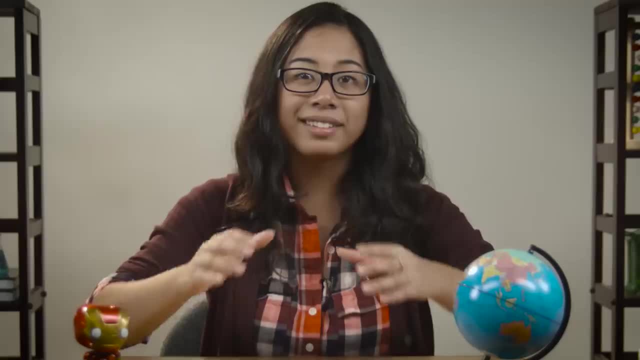 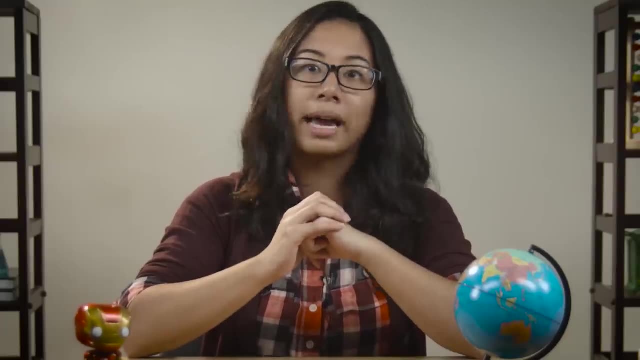 Or I could build a robot that would go down there for me and bring it back. Now I don't want to go down there. It's dark and scary and the potential for getting sewer water on me is way too high. Next, 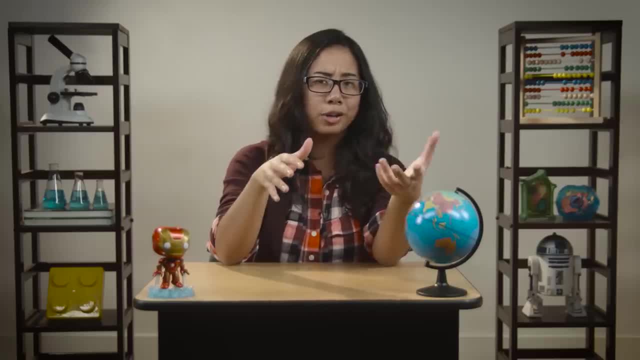 What about using a fishing pole? I think my phone will be hard to pull up with a hook. Plus, I won't be able to see where I'm aiming the pole. It seems like this option isn't the best What's left? 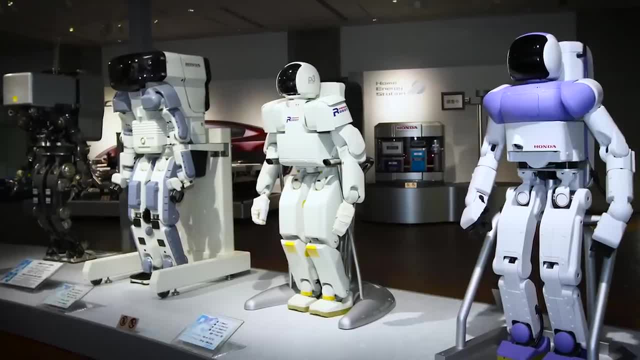 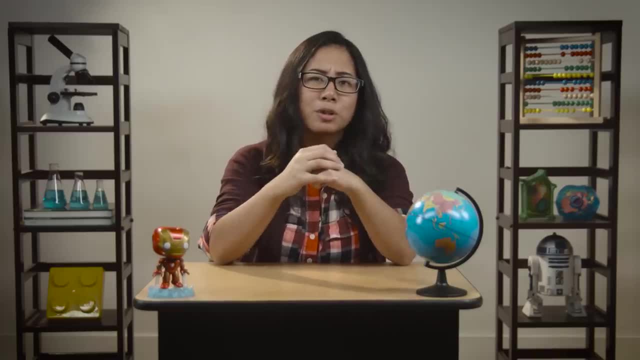 Oh yeah, the coolest option. Robots are used to do tasks that people can't or don't want to do, and that means a whole lot of robots are being designed for this sort of thing- not retrieving phones from storm drains, maybe. 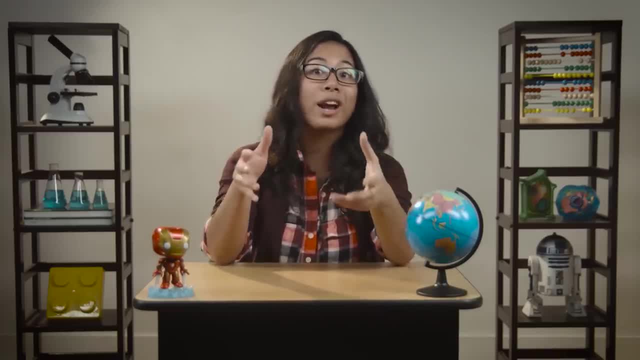 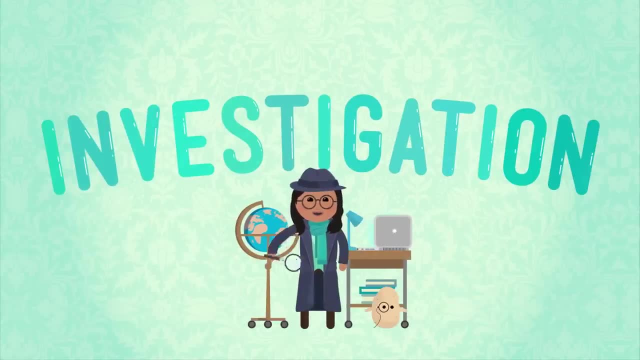 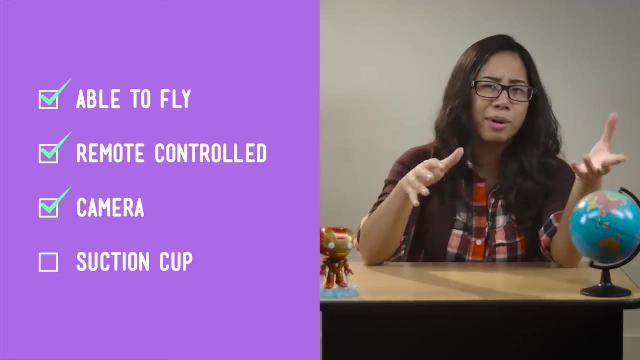 but flying down into caves, exploring the ocean floor and even visiting other planets. So let's engineer a robot. It'll have to be able to fly and be remote controlled And so I can see where it's going. it'll need a little camera. 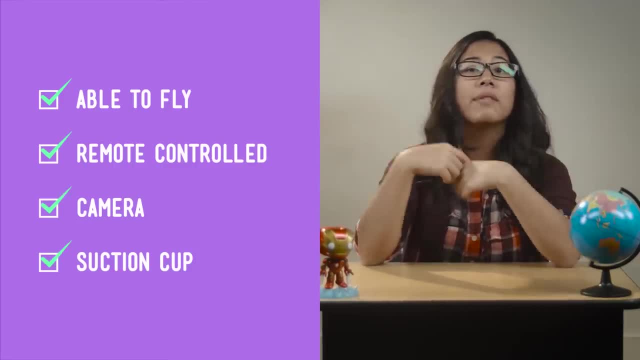 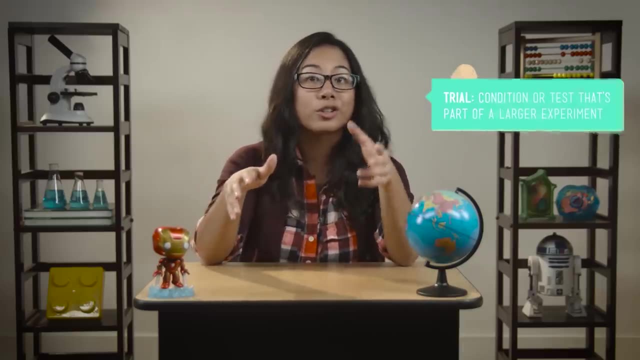 And it'll need a suction cup to stick to the phone and carry it to my loving hands. Now, next, we need to build a prototype that we can use for testing. We need to test or conduct trials in order to ensure success And for those trials to be really useful. 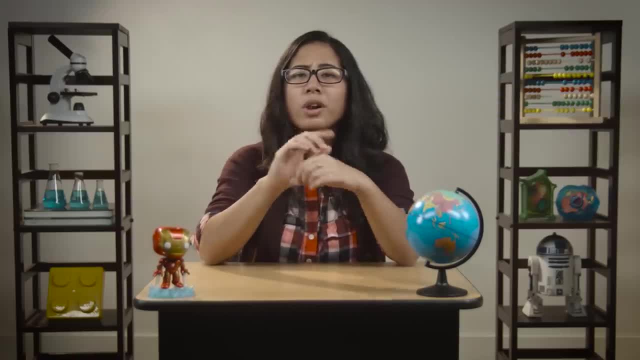 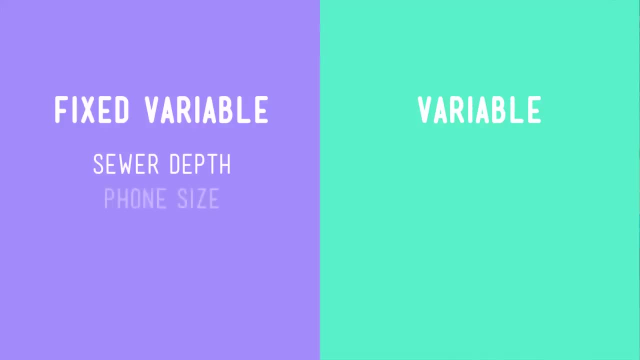 we have to isolate the variables. So what are the variables of our mission? We've got the depth of the sewer drain. That can't be changed, so it's called a fixed variable. We also have the size and weight of the phone. 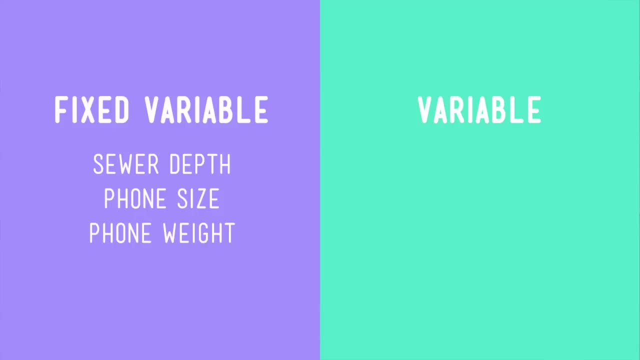 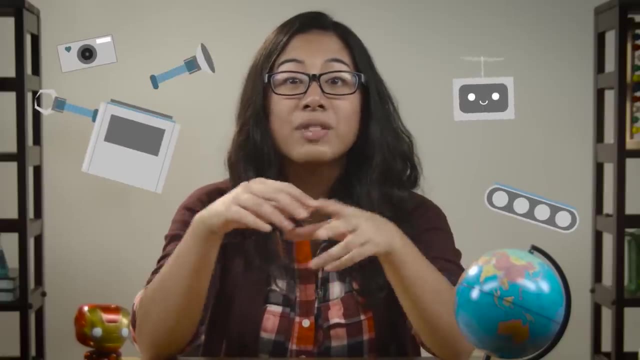 which are more fixed variables. Then we have the pieces of our super cool robot: The propellers, the suction cup, the camera. When we finally get to testing the robot, we need to isolate each of these variables and test them one at a time in pretend missions. 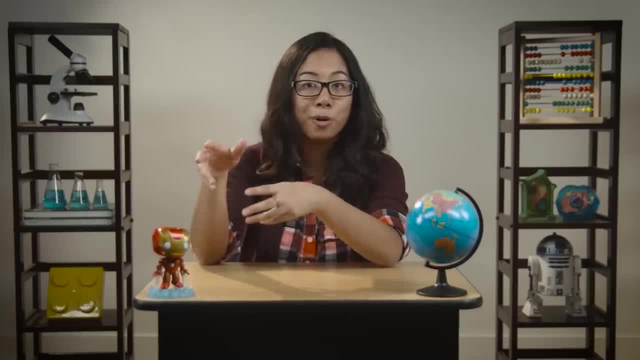 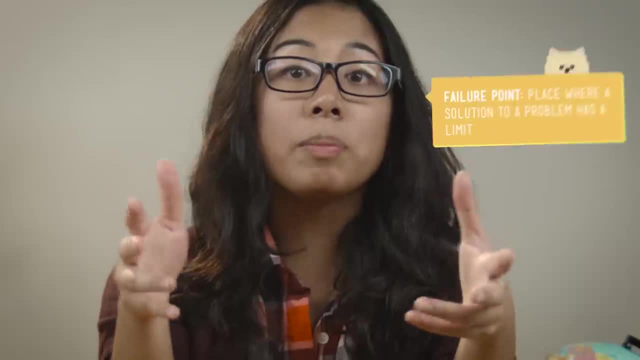 That way we can see which variable we're testing. These variables affect how well our robot performs. Like maybe the robot can carry something the size of a pencil, but it completely crashes when it tries to hang onto my phone. That would be a failure point. 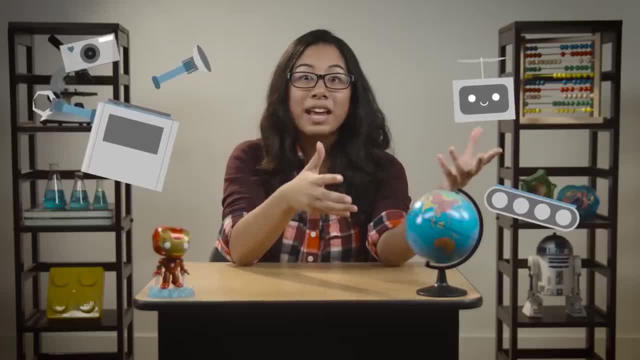 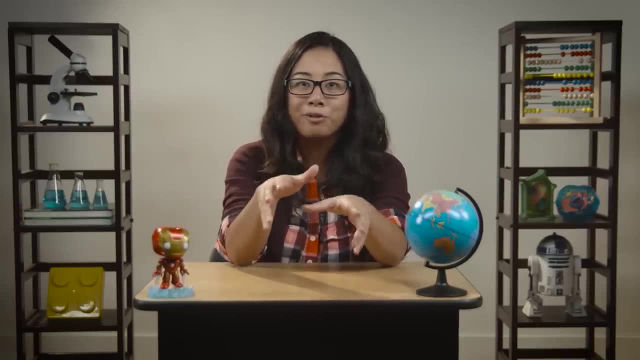 But we can find ways to science around that. If it can't lift something as heavy as my phone, maybe we can make the propellers bigger. Either way, we'll keep tweaking the variables until we get the outcome we're looking for. Then it's all systems go. 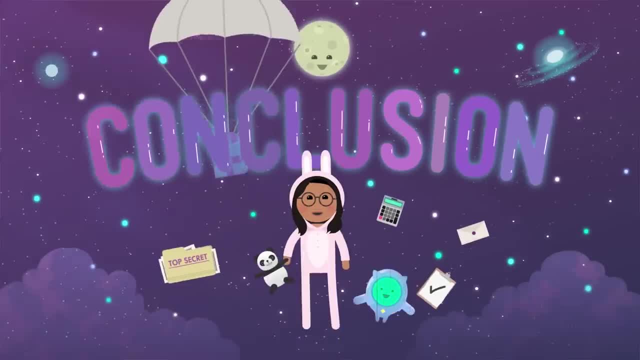 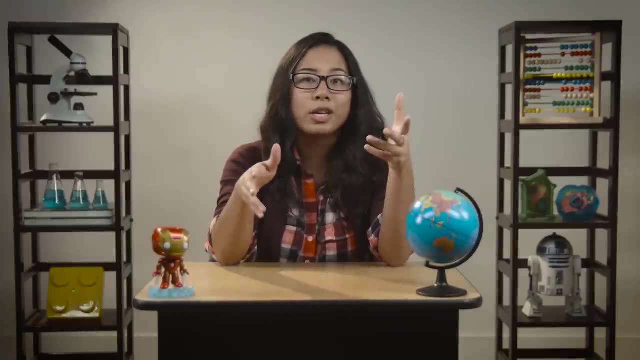 hang on wet and smelly phone. here we come. Today we had a challenge. We had to retrieve something from a deep place we couldn't see, And we had to deal with various variables to find a solution, Variables like the depth of the drain. 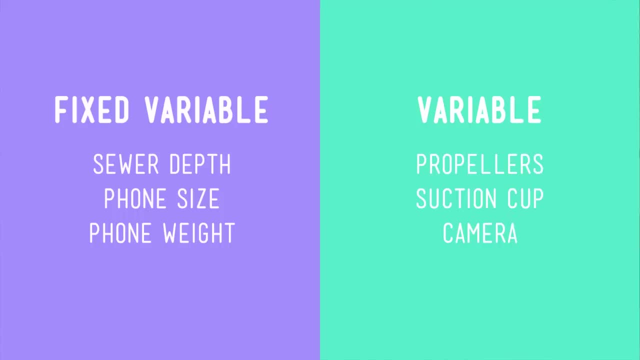 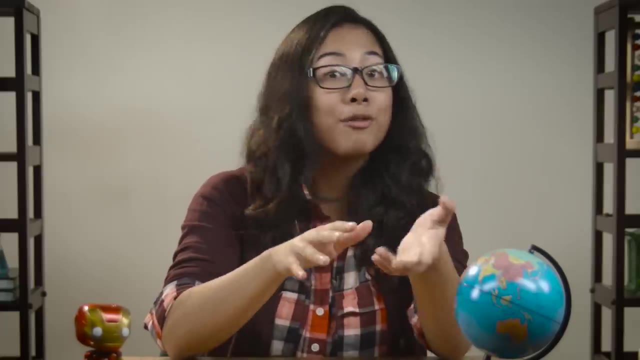 the weight of the phone and the strength of the propellers that made the robot fly Together. we came up with a pretty awesome design solution, But, like I said before, there can be lots of different successful solutions. So here's your challenge. 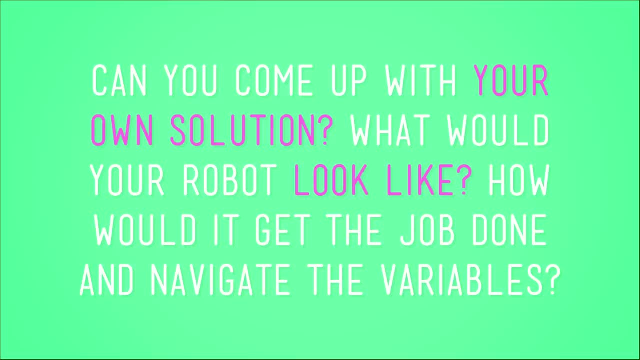 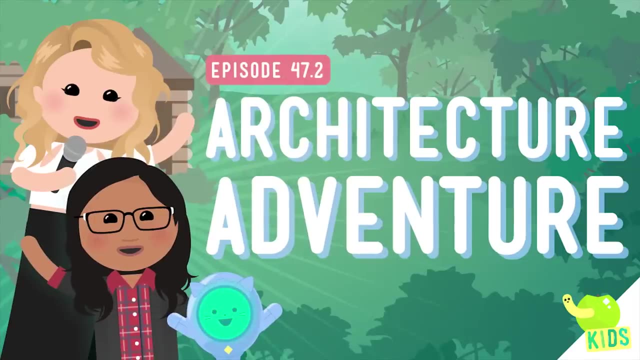 Can you come up with your own solution? What would your robot look like? How would it get the job done and navigate the variables? Put your brain to work and see what you can come up with. I just want to thank you so much for helping out in the last episode. 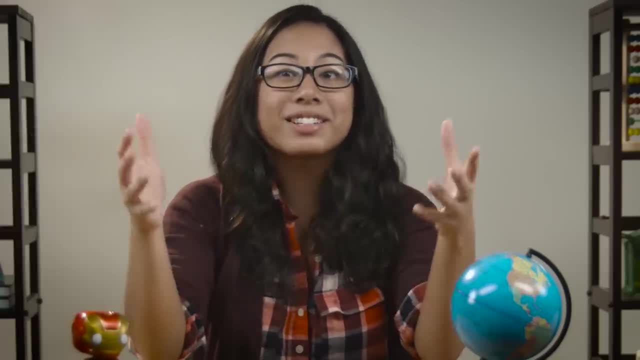 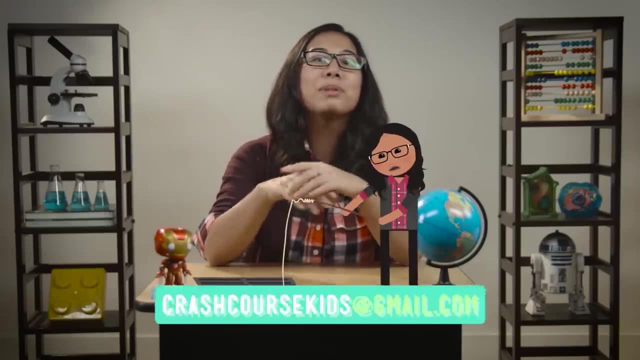 I needed to get my phone out of the storm drain, and together we designed a solution. Our robot was just one of many possible solutions, And maybe you had an even better idea at home. If you did, please send it my way. I'd love to check it out. 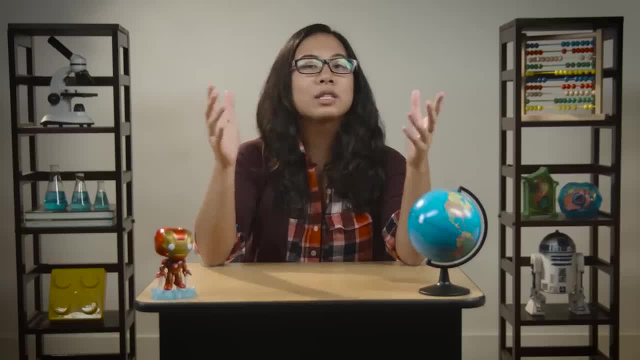 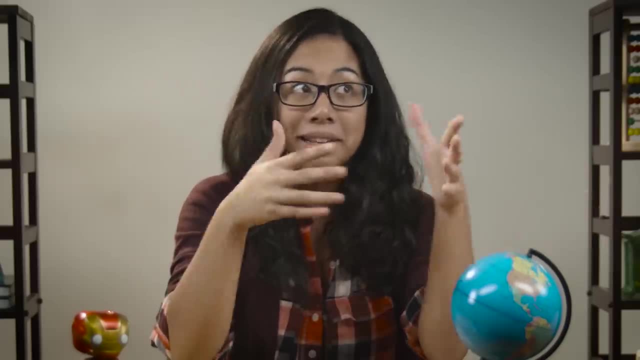 But I've got a whole new challenge for you. Have you ever just wanted some space to yourself, A place to relax? do your own thing, eat Nutella straight off your fingers and burp with abandon? Yeah, I need that. That is a thing I need. 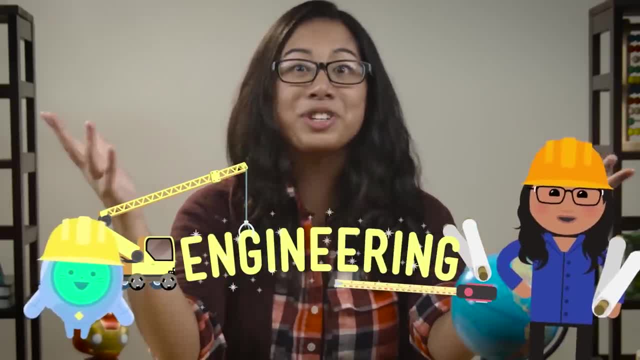 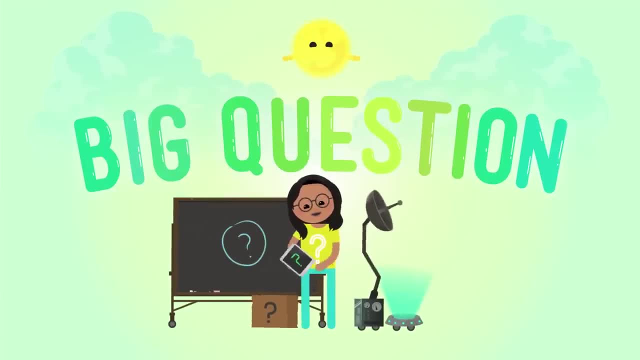 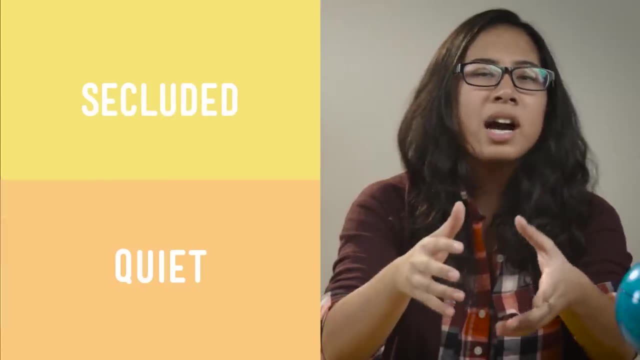 You know it can help. I bet you already guessed it: Engineering. So how do we use the engineering process to solve this problem? Well, first we've got to define the problem. I need a place that is secluded and quiet. I need it to provide privacy and a sense of my own-ness. 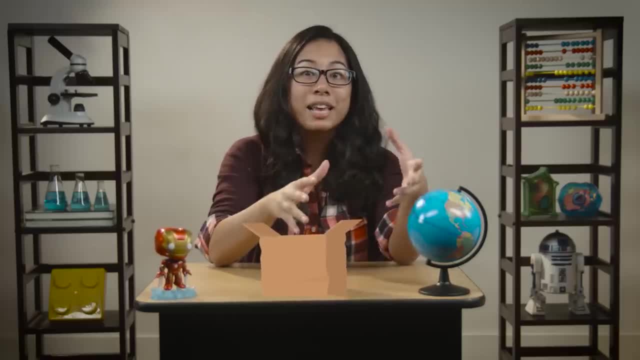 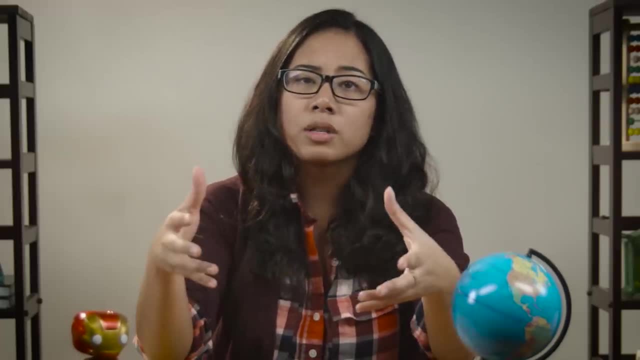 Sounds pretty great, right. What about a big box to use as my space? It's secluded and it can be all my own Solution. wise, it's a problem. That's a start, But a small one. We need to consider more options. 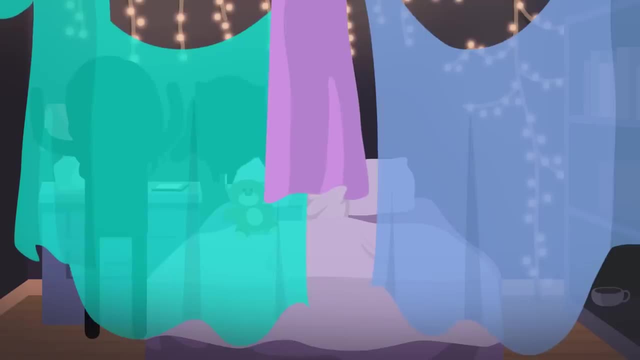 What if I made adjustments to a space? I already have My room. I could hang blankets from the ceiling to help block out sounds from outside, And then I could also sing my head off to T-Swift if I wanted to, without bothering the rest of my family. 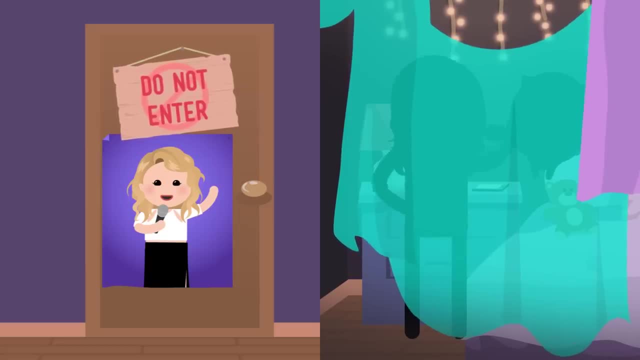 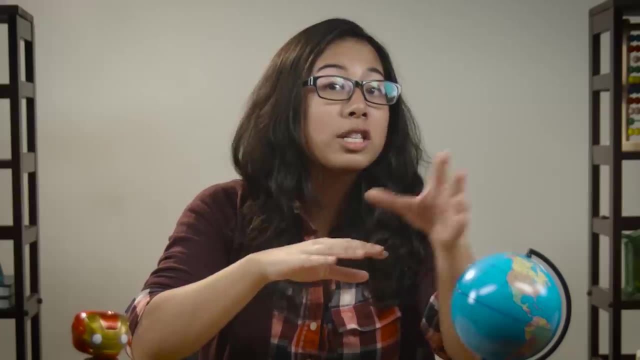 To top things off, I could add a DO NOT ENTER sign to my door, like a serious sign, bold font, all caps: RESPECT MY SIGN. Okay, we've got two options. What else? What if, instead of adjusting a space I already have, I create a new space? 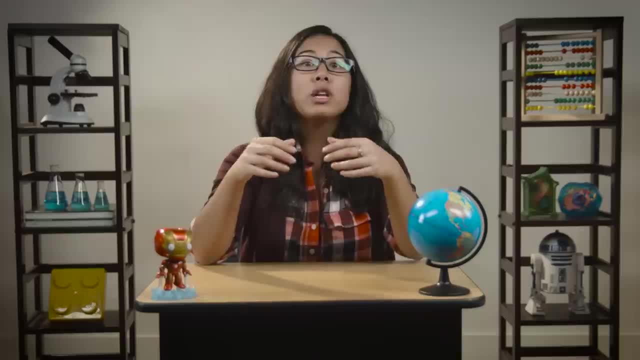 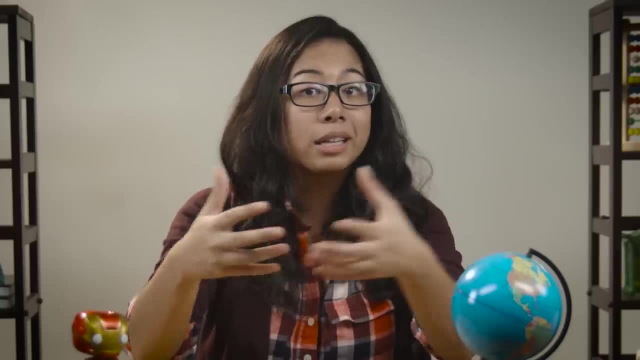 There's a word for what we're talking about here: Architecture. Maybe we could become not just engineers, but architects- Engineers who design buildings. Even though the title of the job is a little different, the process is still the same. So before doing architecture, we've got to weigh our options. 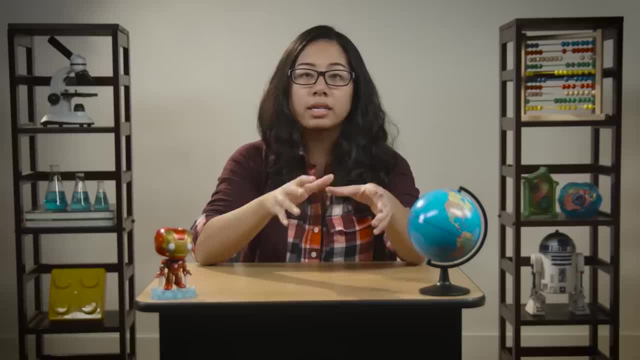 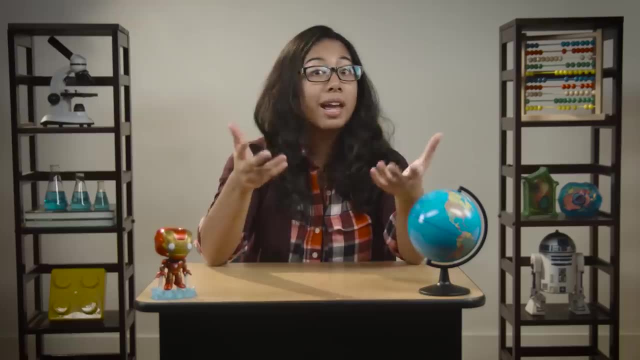 and choose the best design to take into trials. Let's think about the box idea first. It's probably too small. I'd either be squished or be half hanging out of it. Okay, how about tricking out my room Again, while I'd feel like I have a sense of privacy? 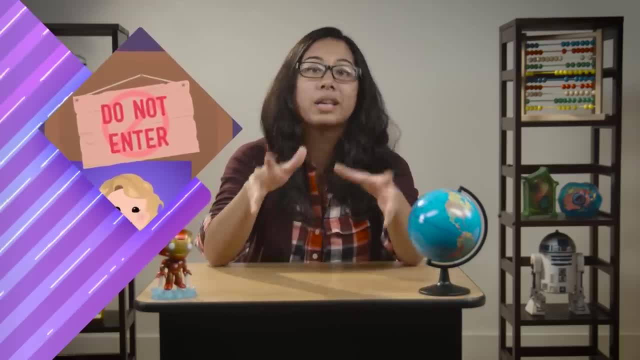 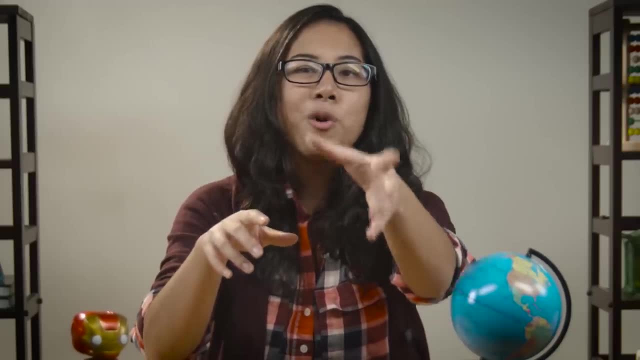 I'd know that at any point any one of my family members could bust in And the blankets on the walls would muffle some of the sound but wouldn't totally block them out. But hey, here's an idea. What about a treehouse? 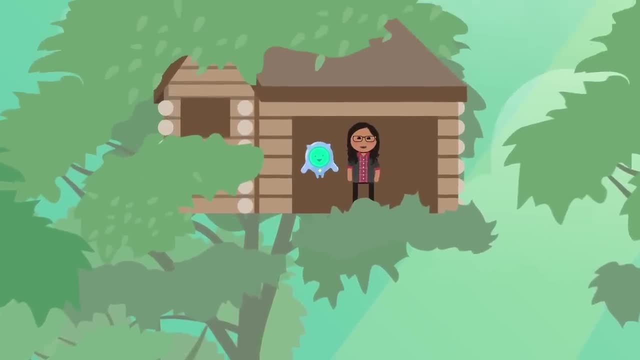 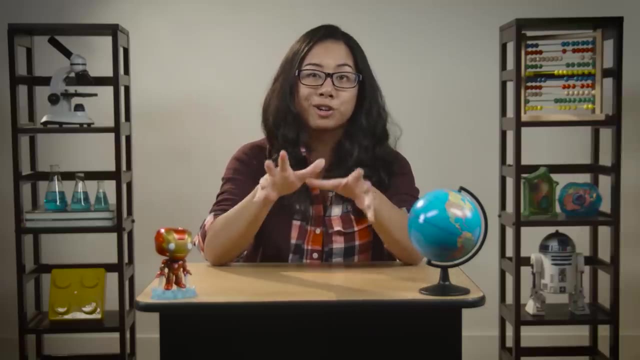 It would be totally my own. It would be far enough from my house that any weird burps or loud renditions of shake it off wouldn't bug my family. Of course it would take some work, Some architecture work. So architect activate. 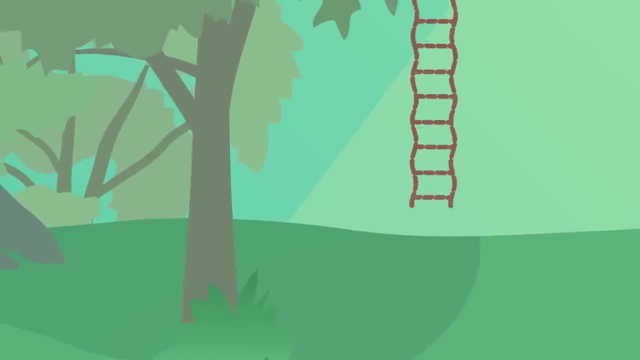 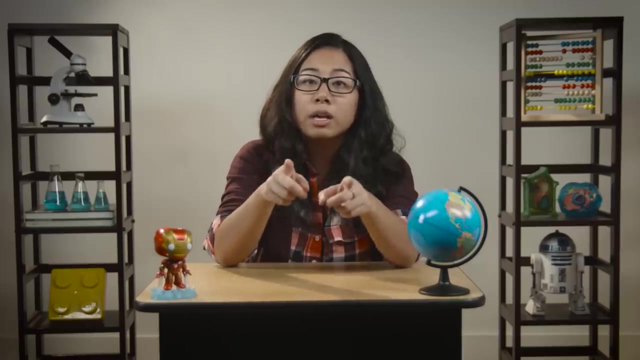 Let's build the treehouse. It'll have a drop-down rope ladder that I can pull up for optimal privacy, And it'll have windows so I can spot when someone's on the way over and properly prepare myself. I can even use the blanket wall idea for my second proposal to muffle the sound. 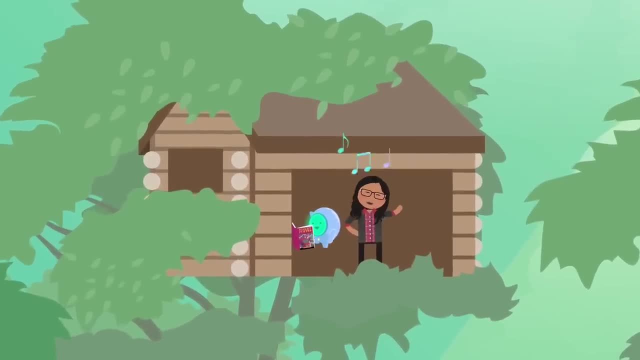 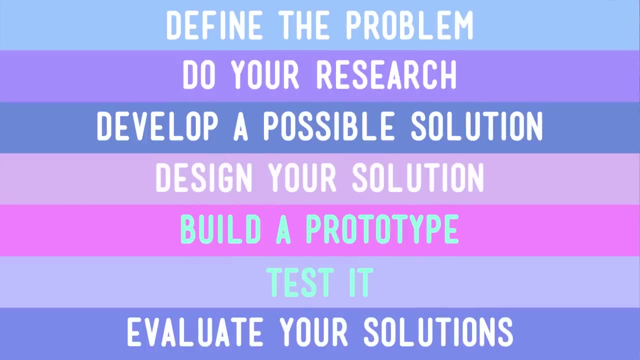 Of course I'll need space for lounging and reading and dancing around. But before we start building, you know what we've got to do: Build a prototype and test it, And in order to conduct useful trials, we need to isolate the variables. 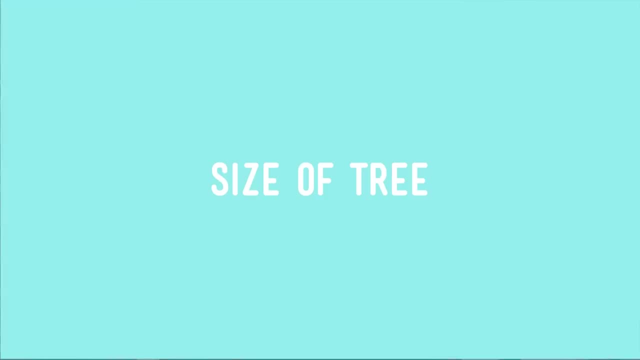 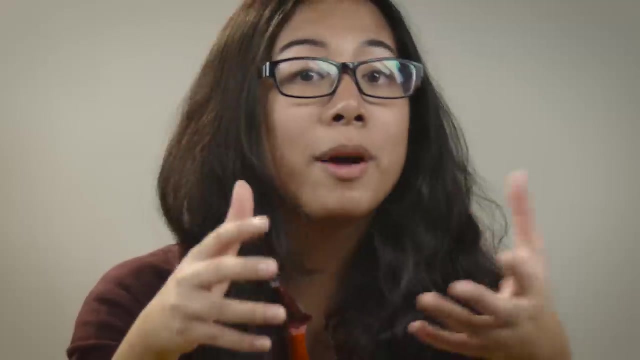 What are the variables of this particular mission? The size of the treehouse we choose and the weight of the treehouse are really important variables, because we gotta make sure the treehouse can stay in the tree. What about variables when it comes to soundproofing the thing? 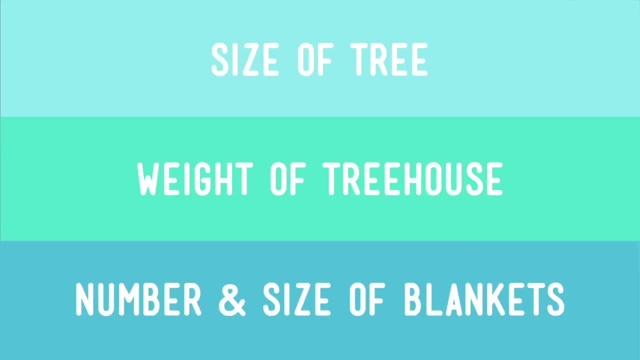 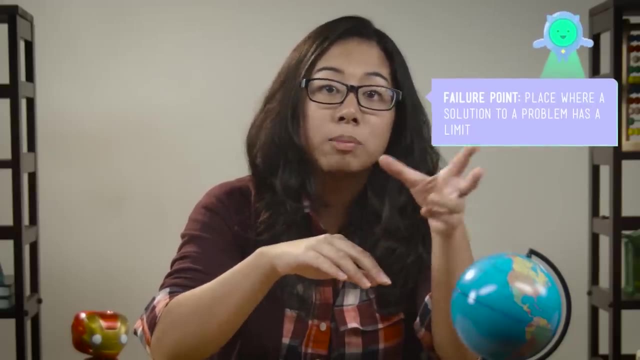 The number and the size of the blankets that I use would be one, and so would be the amount of noise I plan on making inside the treehouse. And we have to keep in mind failure points too. Like the tree might be able to support little old me in a small wooden treehouse.